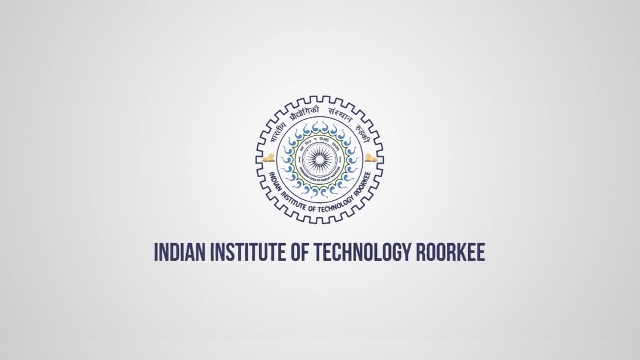 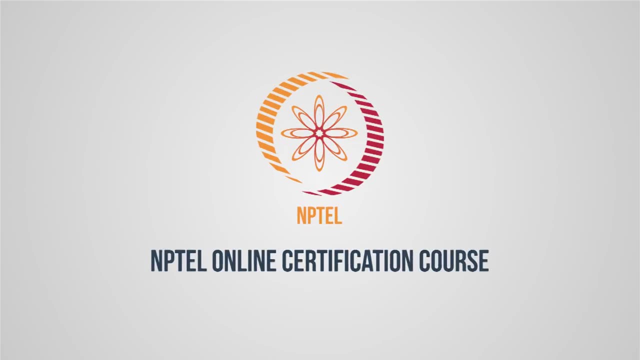 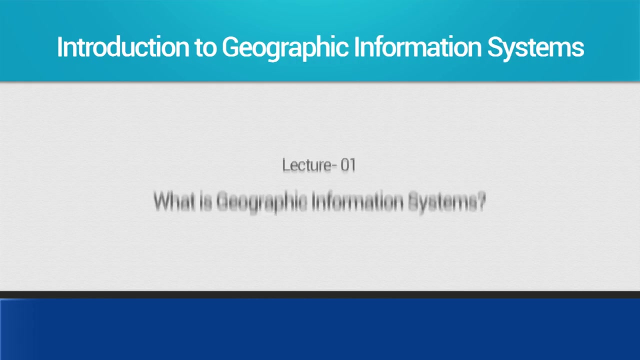 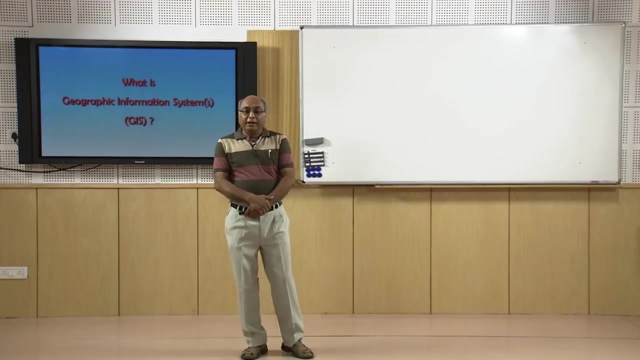 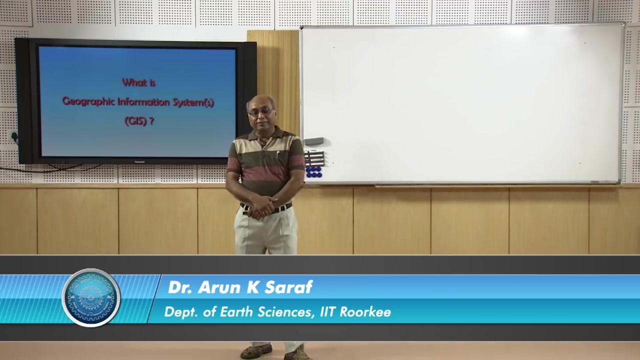 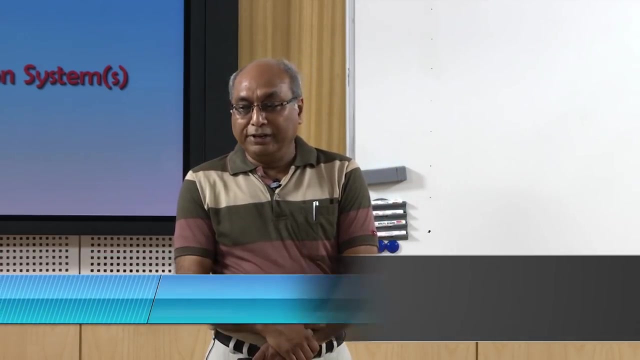 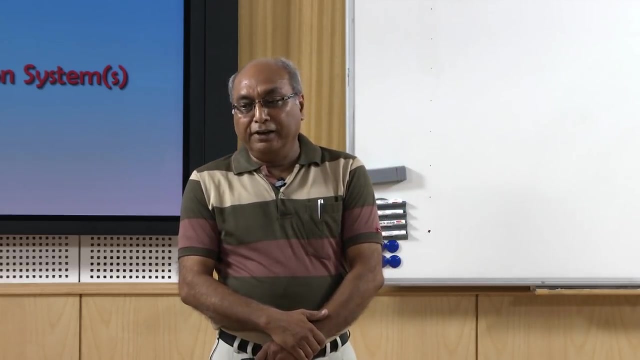 Welcome to this introduction of GIS course. In this course we will have 20 lectures and we will be discussing, starting from, basically, what is GIS. We will go through the definition of GIS, different components and then, later on, all integrations and analysis part of GIS, which is the main important part. 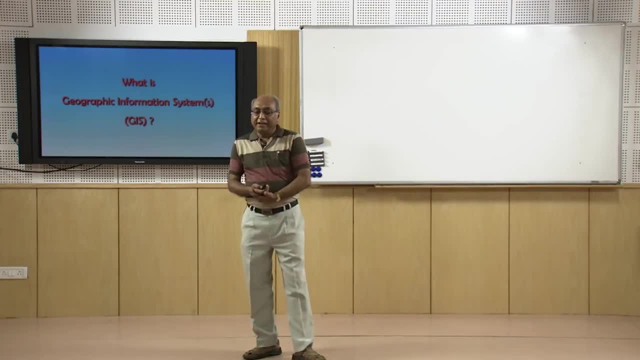 As you can see that on screen, that GIS is made from 3 terms: One is geographic, another one is information and third one is systems. I would like to spend few minutes on the word term which is geographic. Geographic basically does not mean say geography, but geographic. 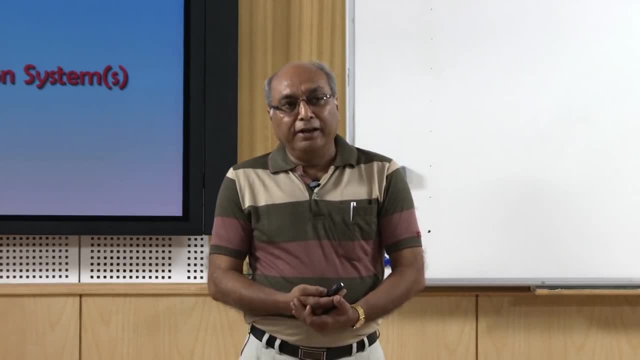 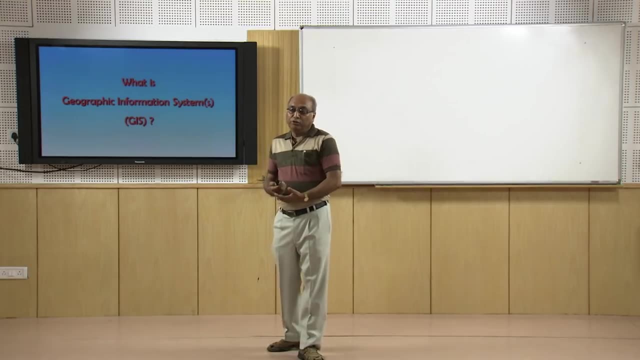 means, say, location, specific data And any object on the earth can be defined or can be associated with geographic coordinates, which we know as latitude, longitude. As we know that entire earth is long, We can have imaginary grid of latitude, longitude and therefore each object on the surface of 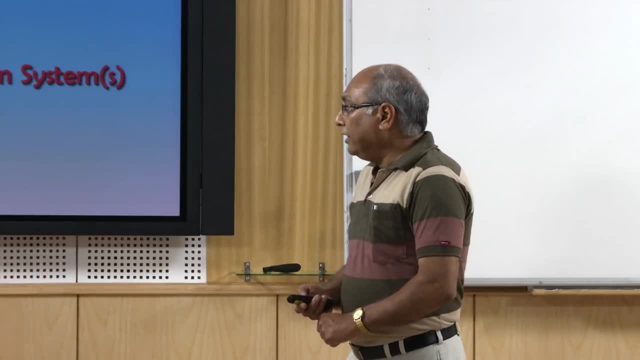 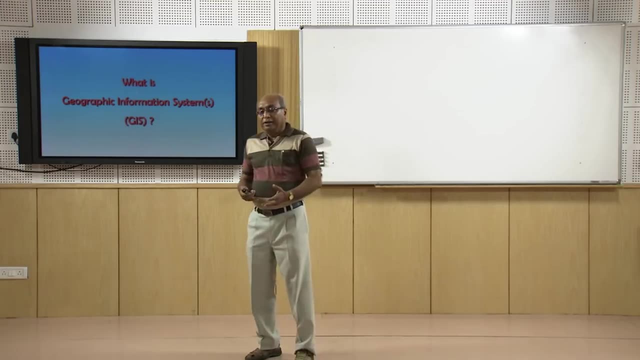 the earth can be assigned these coordinates, And the advantage with the geographic system is that we can not only assign the coordinates, but we can handle very well all kinds of maps and all kinds of data which is associated with geographic coordinates And also another term is used for geographic is spatial. Most of us are aware about the. 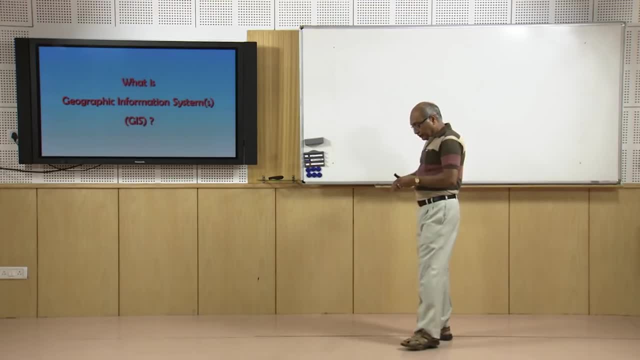 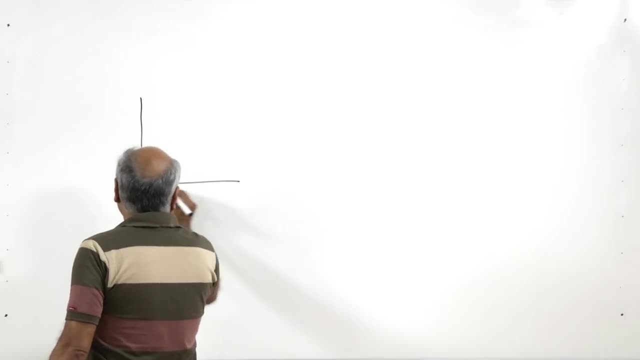 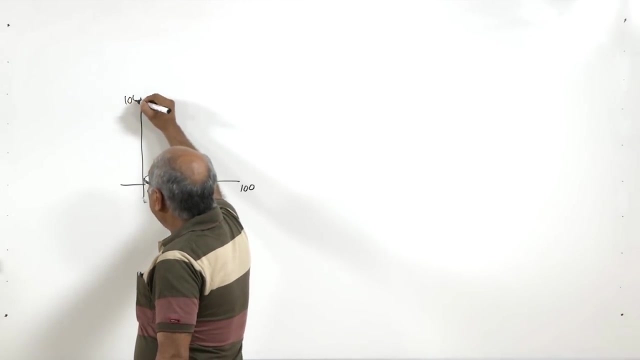 coordinate system, which is called geometric coordinate system, and we have studied coordinate geometry as well. What happens in coordinate geometry? that generally you are having 0, 0 here And then you are having, say, 100 here and 100 here. but once, if I want to do something, if there is a line, 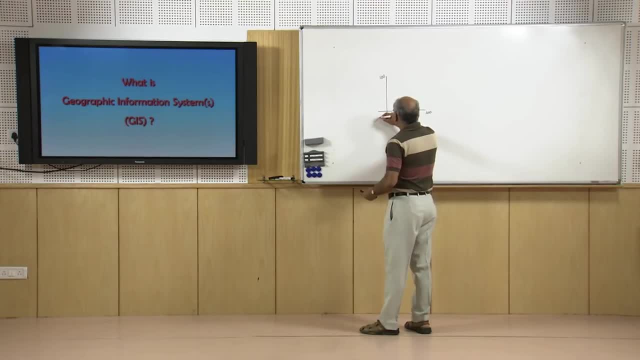 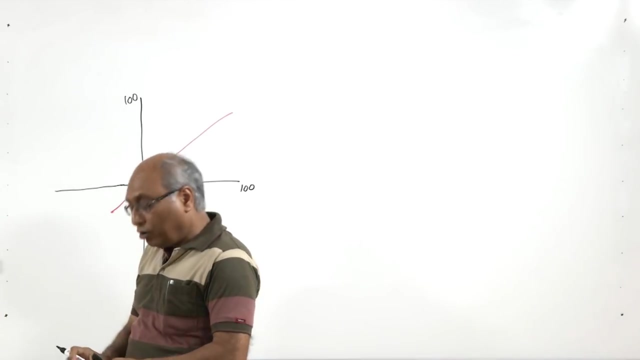 which I want to map, What is the line which is which is going through something like this? and if i want to measure the length of this line, then some part of this line will go in the negative coordinate system and later on it will be very difficult to calculate even the length, or we have to take care lot. 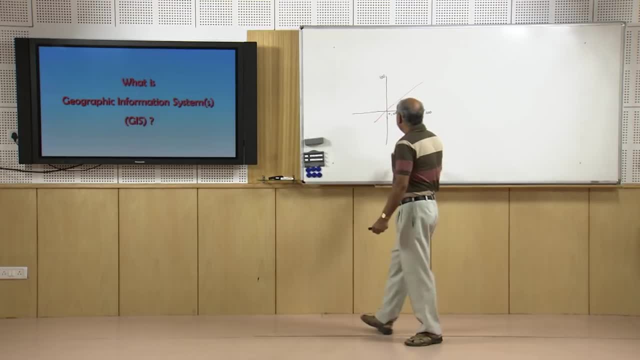 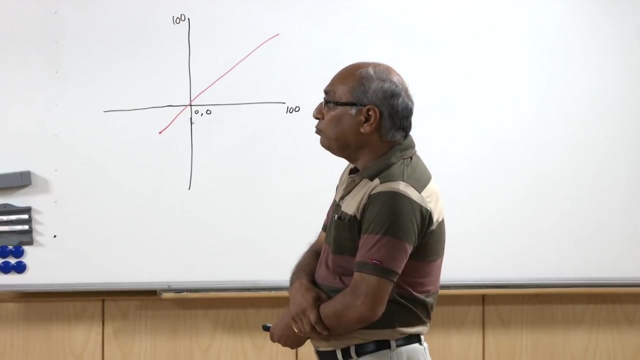 of take care about the length of the line. same would also happen in case of area. but if we handle such data like point line or polygons in your geographic coordinate systems, then this handling becomes much easier. and therefore, ah, this system has been, ah, come into picture and little bit. we will spend some time on the history of a gis and this. 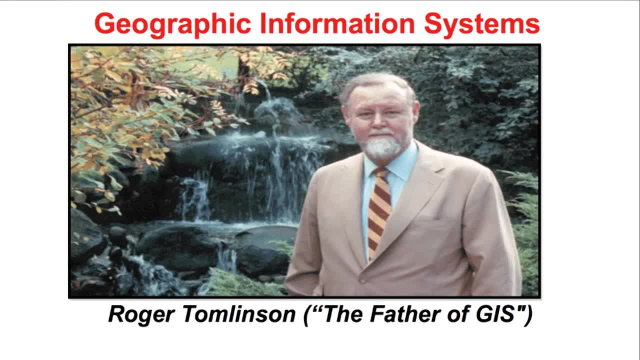 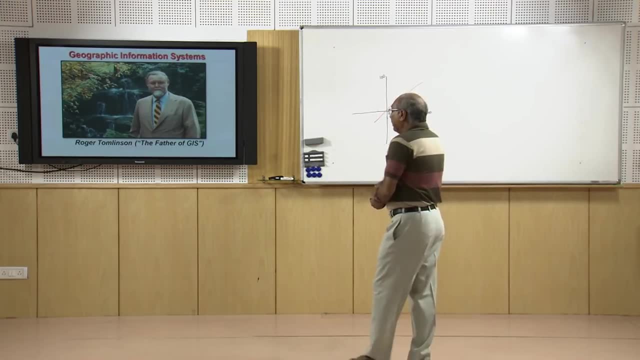 ah, this was the term which was given ah- by a person whose name is roger tomlinson, who is also known as nazi nowadays as father of gis. he is a. he is a computer scientist because he is still alive and he used to work in the canadian center, which was looking after the municipal cooperation. 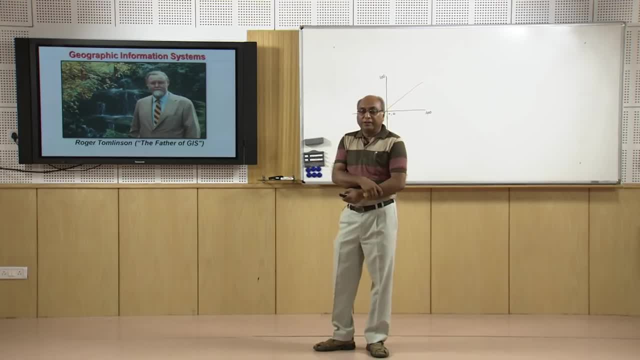 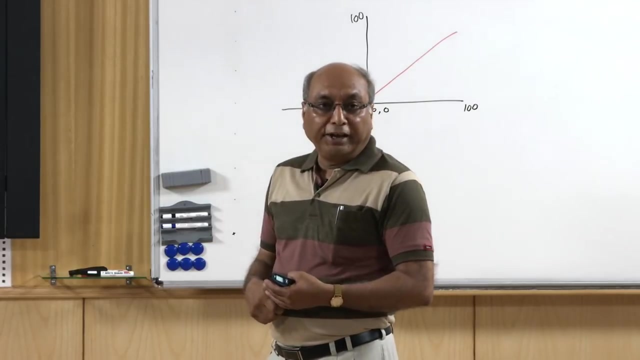 of ottawa and they had lot of networks of say gas pipeline or telephone lines, power lines and road network. so whenever somebody used to go to dig a say gas line, then say gas line and at the same time he might damage the telephone line or electricity line. so 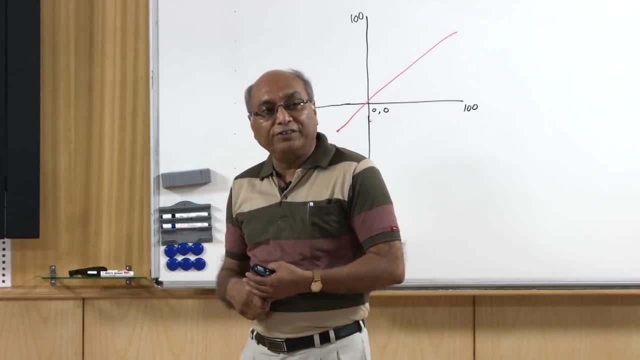 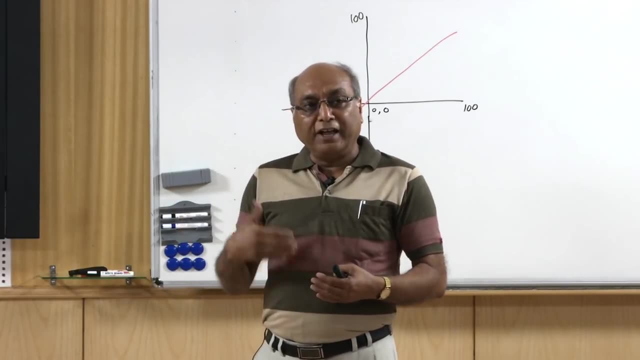 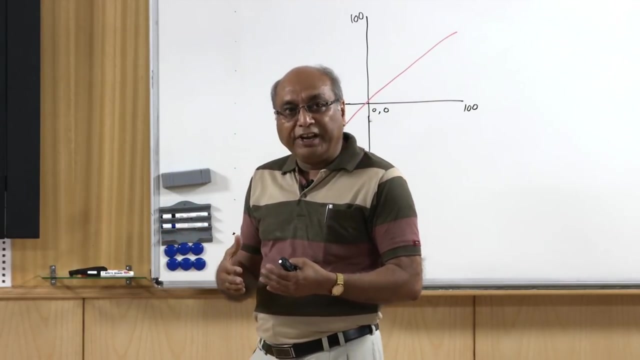 the task was given by the ottawa municipal corporation to this a computer engineer that can you develop a computer system by which a when a person is assigned such repair work, he should know that at what time and at what depth, at what location he will encounter another? 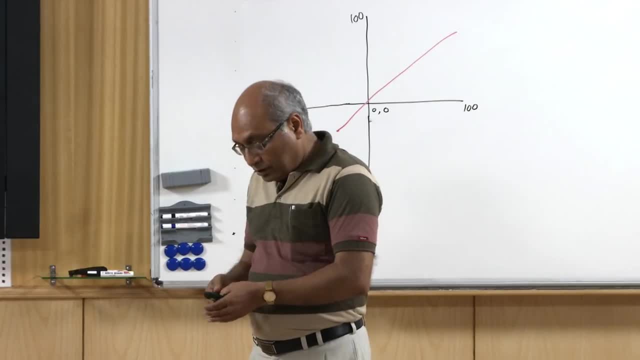 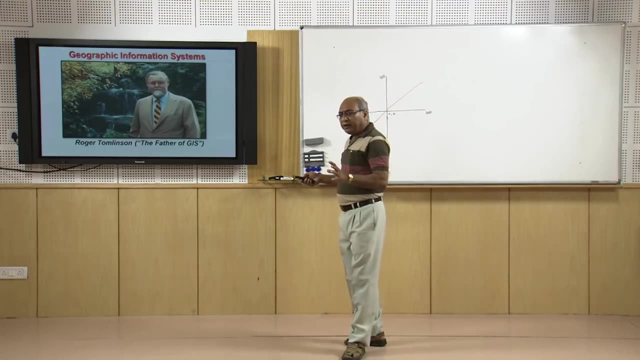 network and for that. then he started working on this kind of concept and he started to and he developed this geographic information system. There are different terms nowadays, are there like many people would like to call as a geoinformatics, which involves not only GIS but also remote sensing, GPS and overall computer technology? 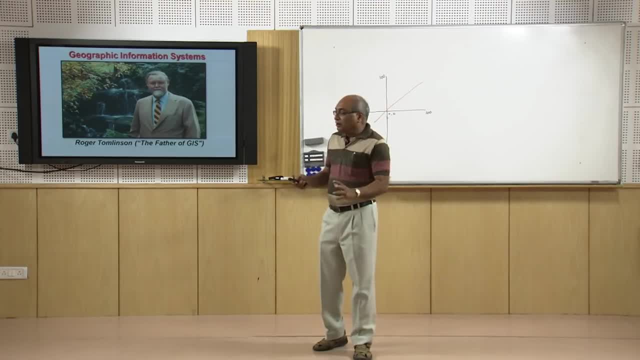 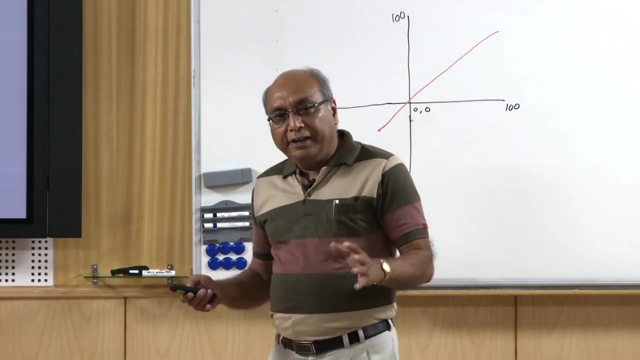 Some people call as a spatial information system, but all will converge on one concept. The basic is that handling the data in geographic domain rather than in geometric domains. That is the main difference here. As we know that there earlier there are still exist some CAD CAM systems in which a geometric 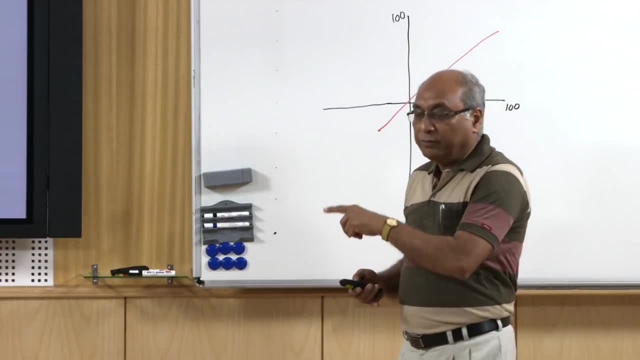 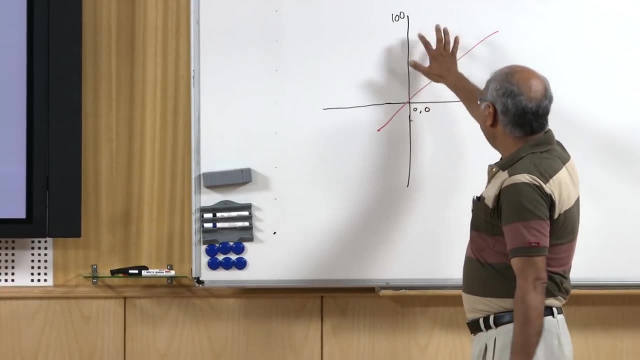 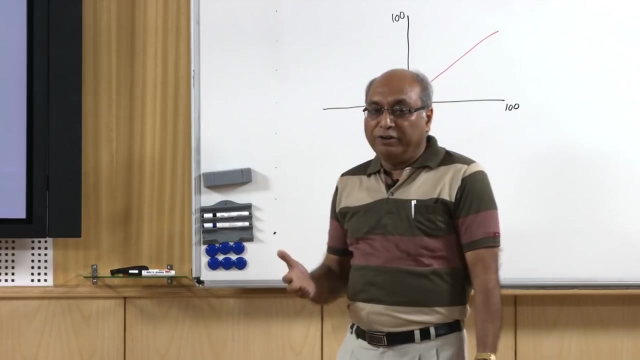 coordinate system is used, not geographic coordinate system, And therefore there are some difficulties people encounter, especially when I want to. if I am having a map of this portion, When I want to add another map, When I want to add another map of adjacent portion, I might have difficulty in a geometric 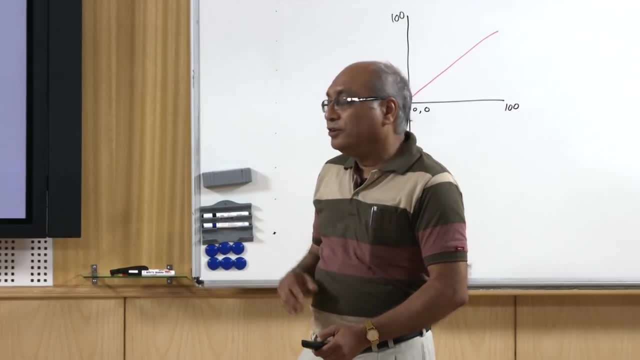 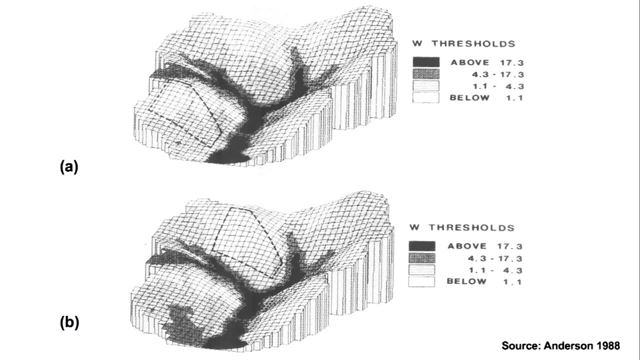 coordinate system, But in geographic coordinate system, such difficulties will not arise. That is the advantage. one of them, Because the main purpose of GIS is not to store the data or keep the data, but provide analysis. and finally, as most of the systems, they provide the platform to model the data. 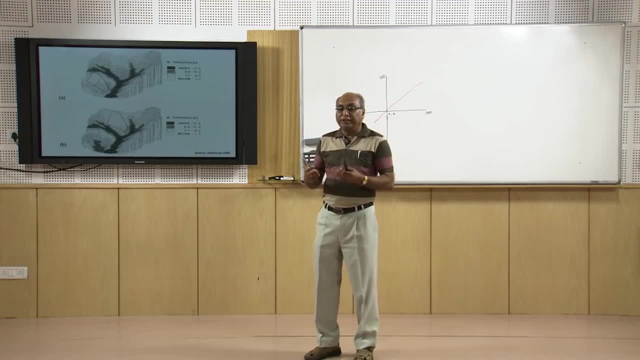 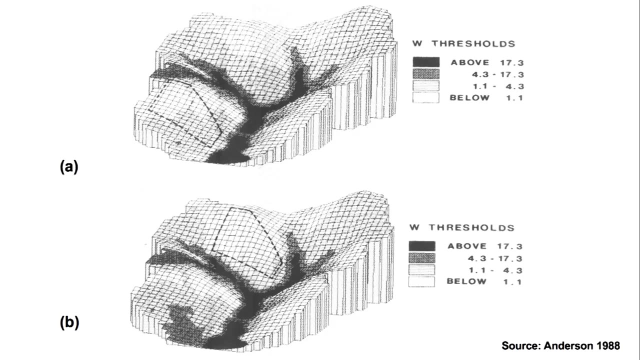 or to use these data. So that is the advantage. You can even use a GUI system to predict something which has not happened yet on the ground. So here I am, showing the same watershed in two up and down, And this watershed, as you can see, the boundary is here, say, showing in a grid form. 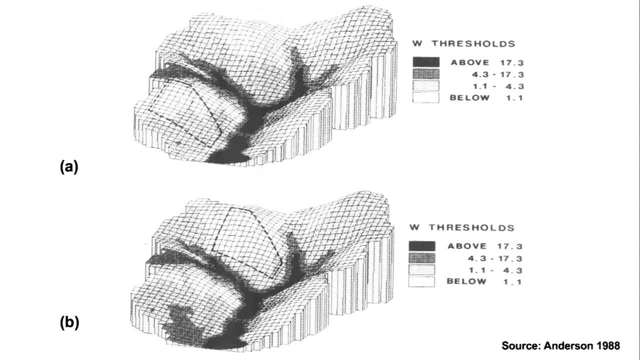 And some this water threshold or in simple terms we can say the soil moisture here. So what we are seeing? that there are different sets here And one, this dash, dashed bracket or an area is marked here and in the same water set the same at another location. 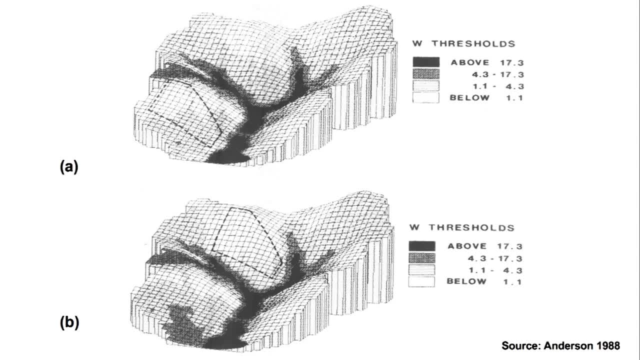 having the same area is also marked. but it is basically indicating that if in this particular water set, if this part, the forest of this part of the water set is removed, then this is going to the scenario of soil moisture conditions. And if same area but at different location within the same water set, if the forest cover. 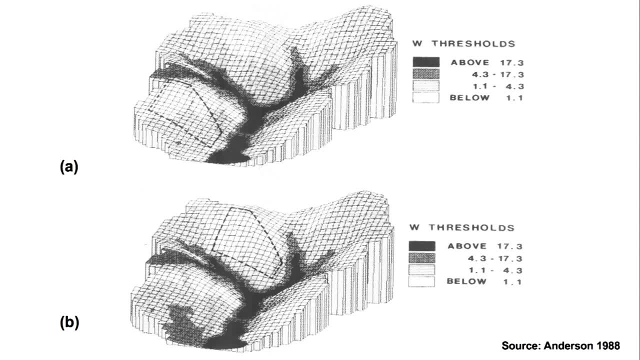 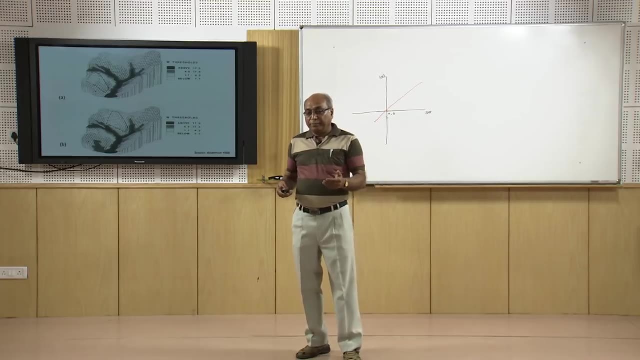 is removed, this is going to be the change in the soil moisture condition. As you can see that here this is bringing all together a new scenario, which is not there in this case. So what, basically, GIS is providing us to predict something which has not really happened. 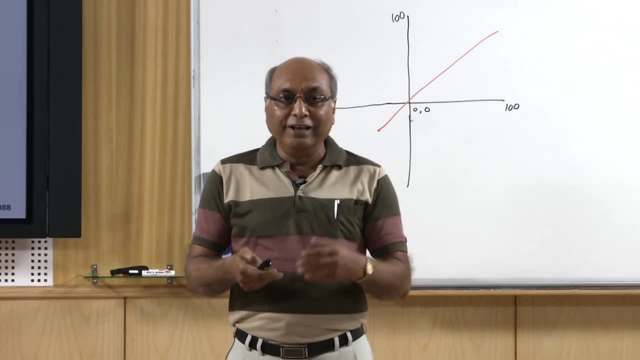 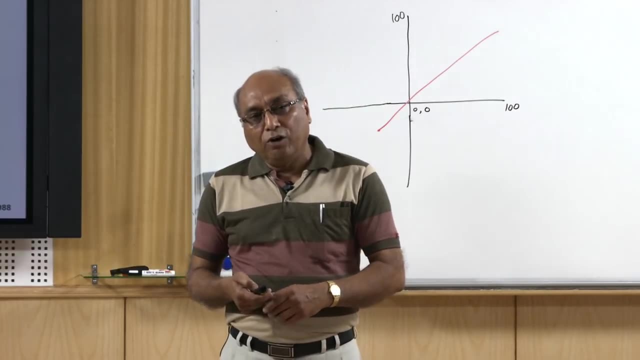 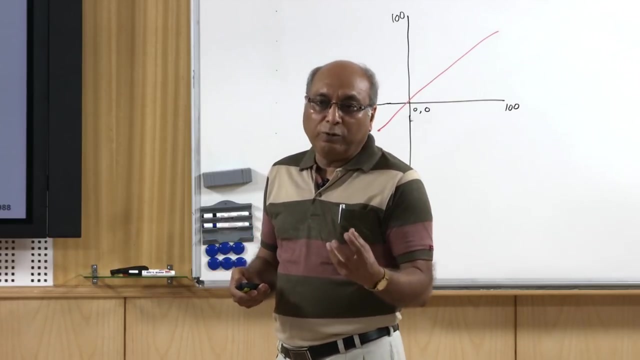 That means you can simulate lot of real things, real scenarios, real problems which are related with nature or complex processes of nature within the computer, before anything really happens on the ground. That is why it has become a very powerful tool for modelling and also for prediction. 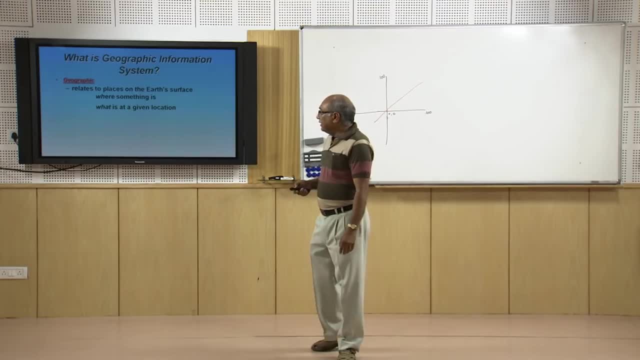 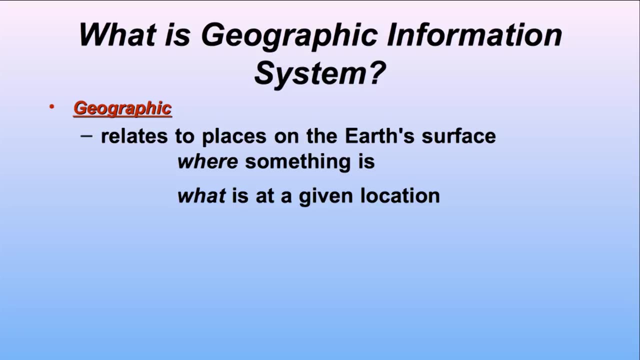 So, as I mentioned earlier that the geographic means it relates to the places on the earth surface And in geographic Coordinate system, not in geometric coordinate system. and then we start answering questions that where something is, because once a location is attached to a object, then we can answer. 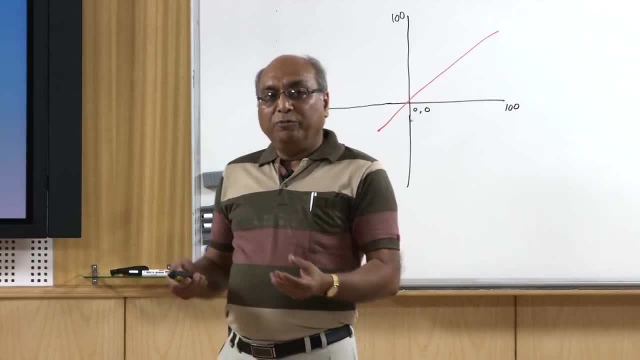 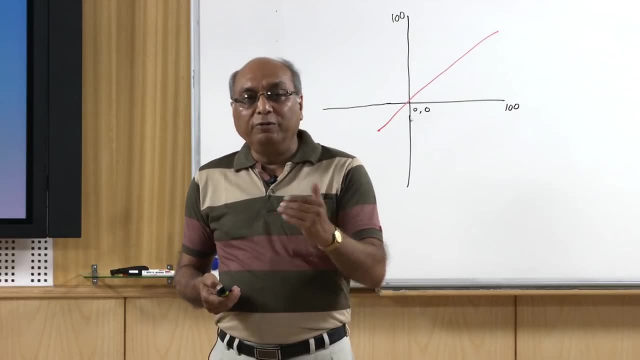 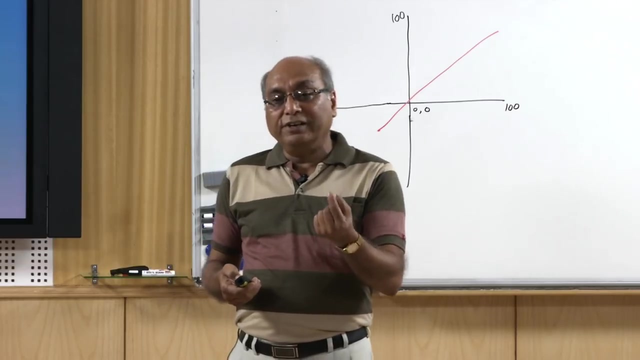 where it is Like nowadays. we know that with mobiles and with the coordinate systems, we can find out, or, very soon, we would be able to track each and every mobile through the GPS, because GPS provides the information, which is the location, Which is latitude, longitude of that particular mobile. 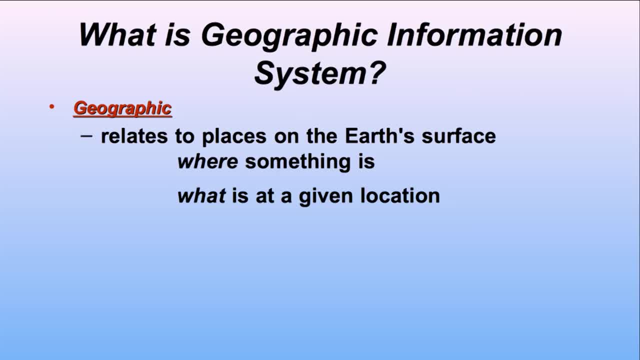 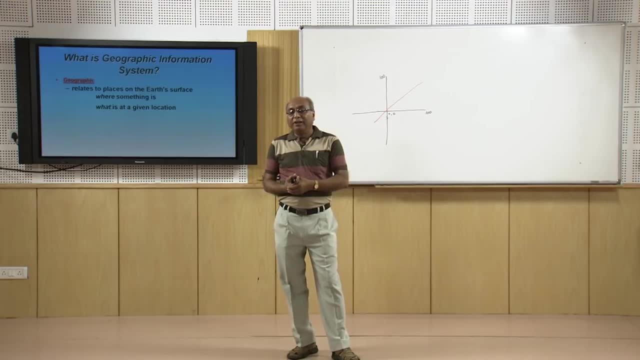 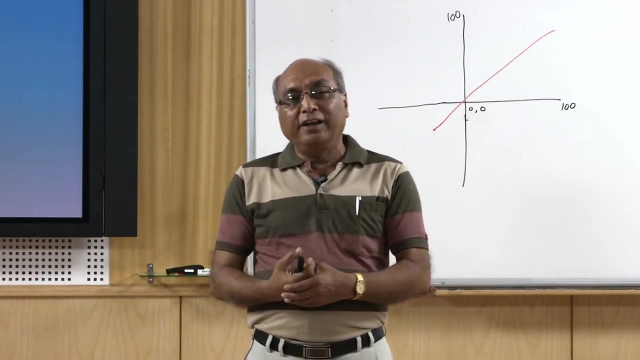 So similarly here that in GIS, we get the information or answer of a question that where is something? and also another question, that what it is giving location. So once we have attached an information, let me give you one very interesting example, Like there are. every year there are GE, examination is conducted, but we keep all this data in. 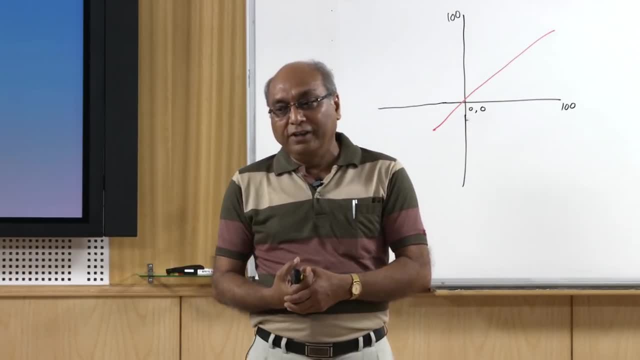 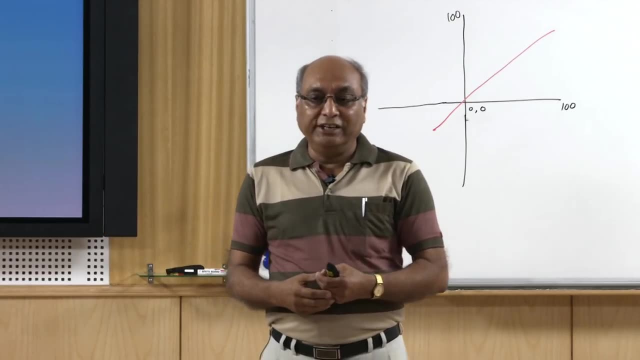 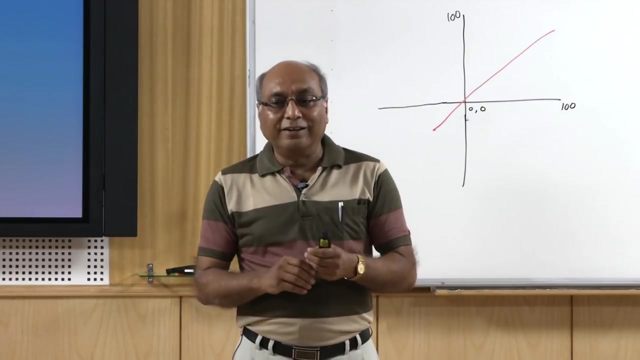 a database. We do not keep this data in a geographic database. Suppose, tomorrow we start keeping the coordinates of each candidate who is appearing for GE in a geographic coordinate system or in a GIS platform, what would happen once the student are selected? then we would. then we will plot this, you know: appeared a student versus selected? 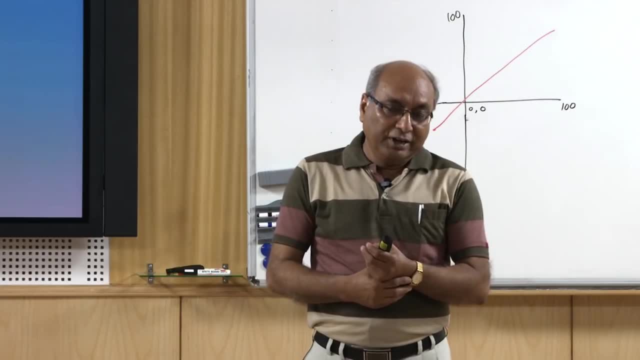 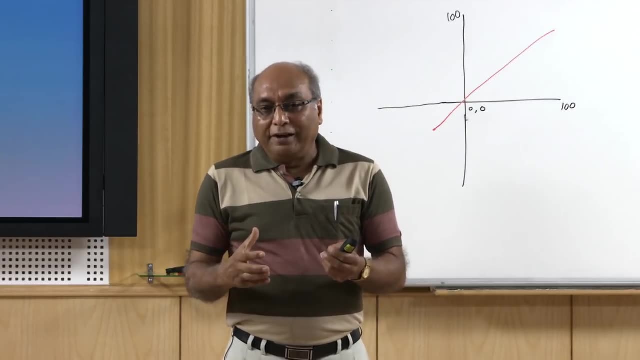 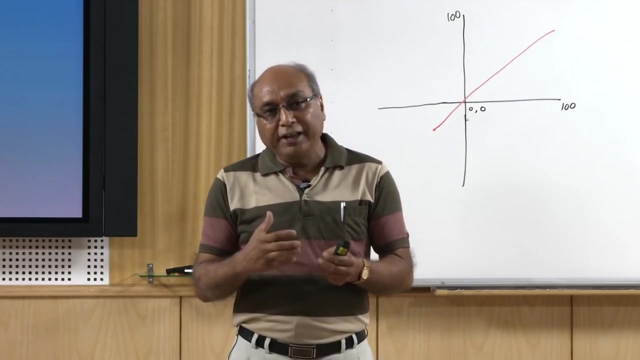 student. We should get a very interesting plots or distribution of the data and we I am sure we will also find some clusters. So clusters will raise the question why it is happening, why not throughout? this distribution of selected candidates throughout India is same. why it is happening in a cluster form. 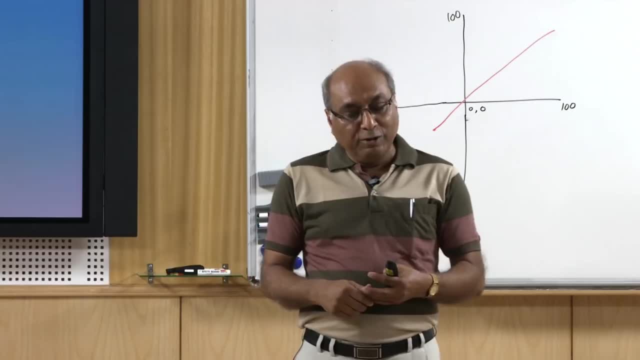 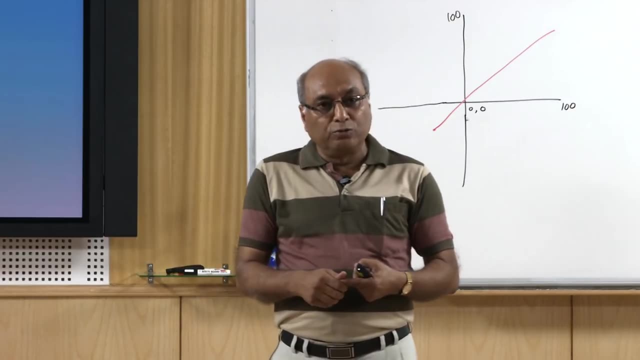 might be because of good coaching, might be the intelligent level of people are higher, or is it related with the you know economic things, or is it related with the schooling? all kinds of questions will come and then we will be able to answer, If we are able to answer. 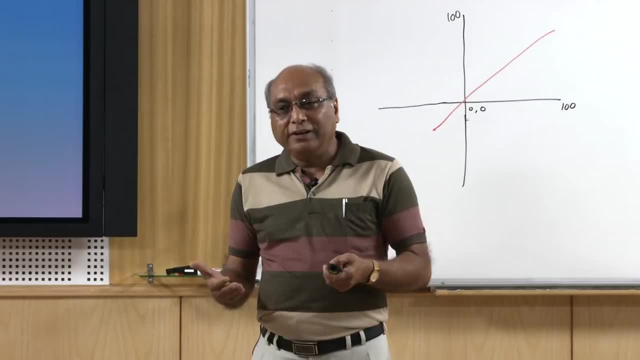 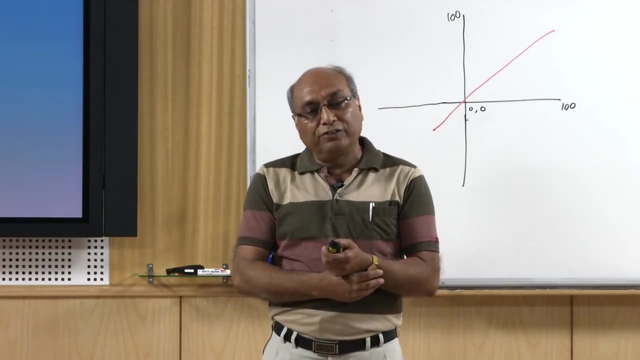 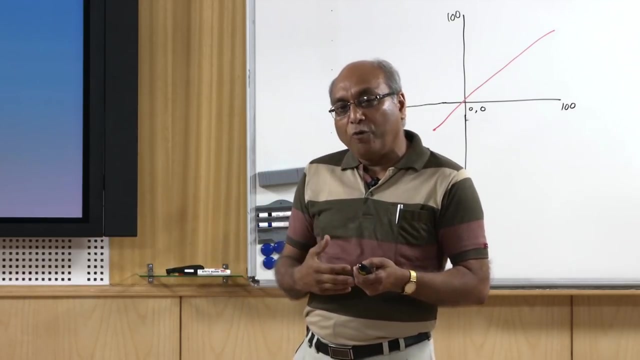 If we are able to answer. If we get few more data, like economic data set or may be schooling data set, climate data set, if we start adding in that geographic system or GIS system, we should be able to answer that why there are clusters. So, similarly, lot of such phenomena can be understood very nicely once we assign the. 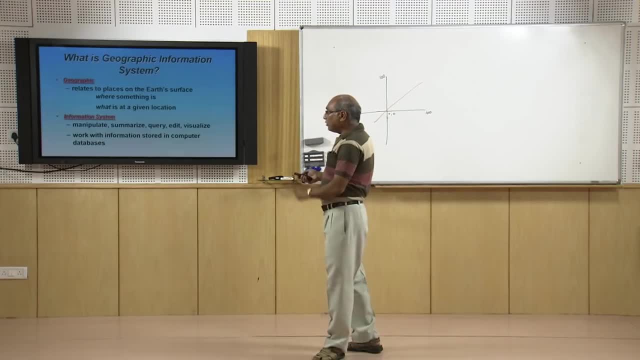 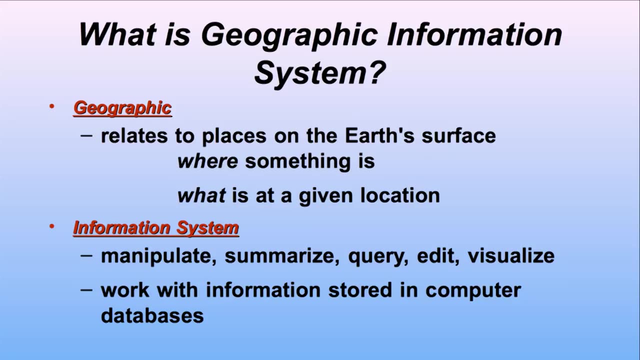 location to certain objects. So that is why geographic world is very, very important. the other two terms which are used, which most of us are familiar, is about information and systems. That information and systems which we- because the data is converted into information through computers and which allows us, which GIS platform allows us, to manipulate, summarize also: we 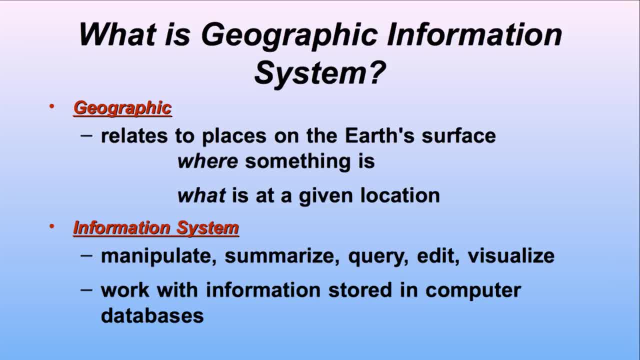 can raise the questions to the system, we can add it, we can visualize. visualization is very, very important thing. the in the previous slide when I have showed the water set, that is also visualization. So visualization before really anything happens. and with the we work on the information or 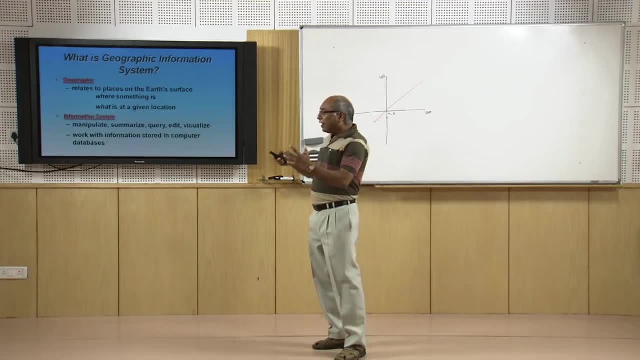 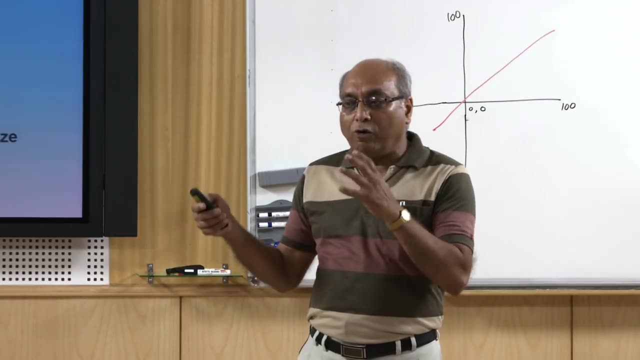 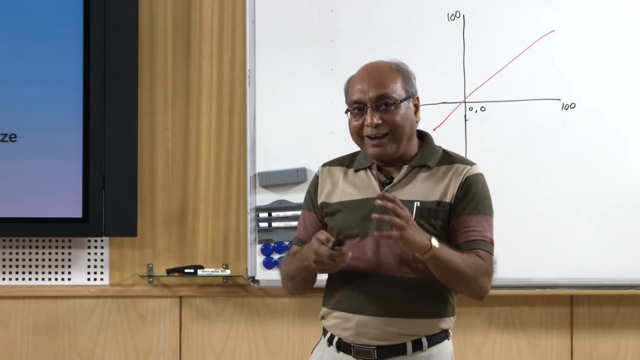 data which is stored in the computer database. So it is a kind of integrated system which is having not only the geographic data but in a database system. So all the qualities of database systems- DVS and DVMS systems- are there and all your CAD systems capabilities are also there. so it is a kind of integrated system. 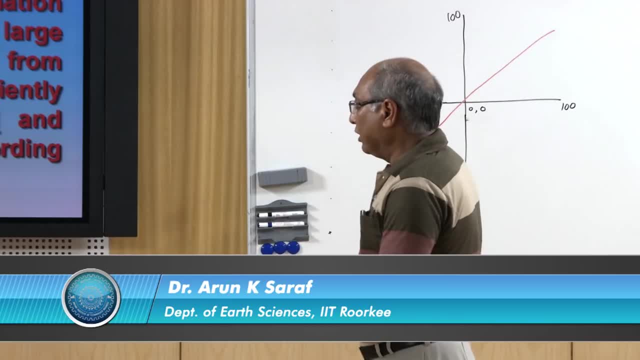 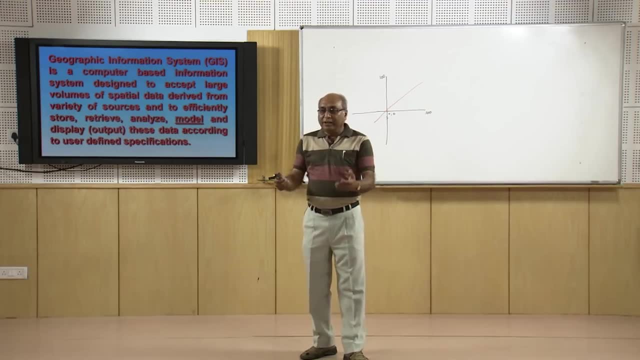 Slowly. We will learn how it is progress when we progresses in this course. So let us have a look on the definition of a GIS. this is a most modern definition of GIS. in different books, literatures or internet you may find little varied definition. 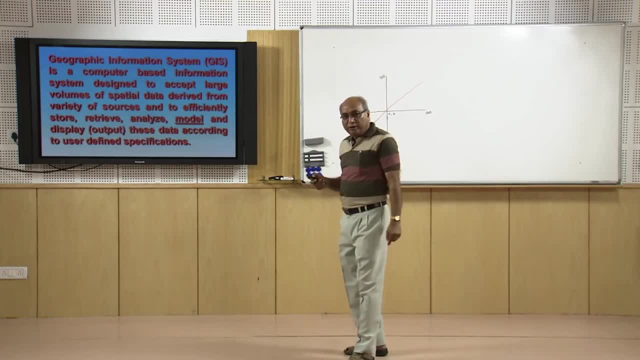 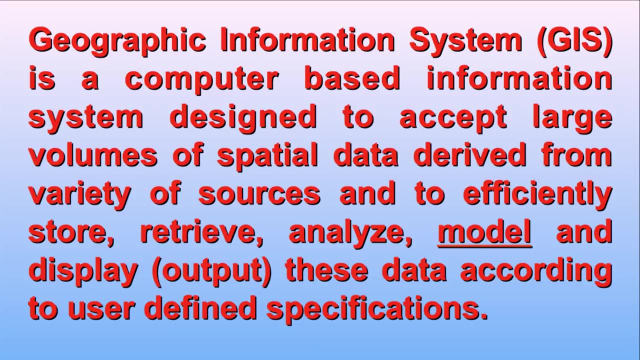 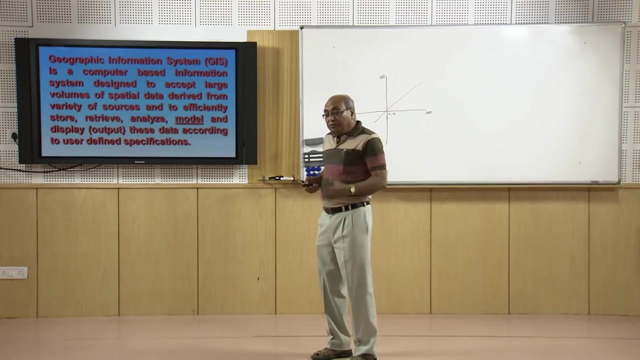 But if we here, each and every word is very, very important and therefore I will go one by one through all these terms or words which are mentioned in this definition that GIS is a Computer Waste Information System, That means that can we have analog GIS system? no, very, very difficult, because earlier when 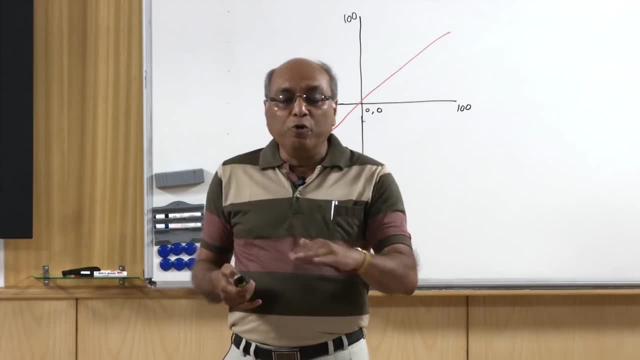 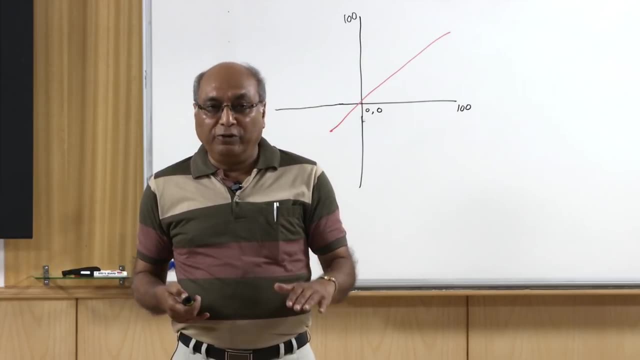 we did not have a good computers, there were people who, who, who, who were having some maps or data in a transparent sheet or tracing papers. it was very difficult. So manual system of GIS is not really possible and that is not really truly a GIS which present. 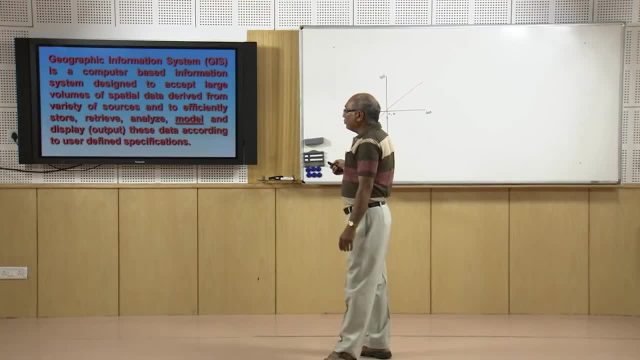 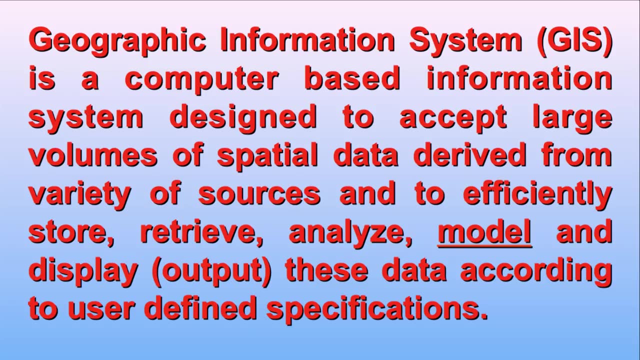 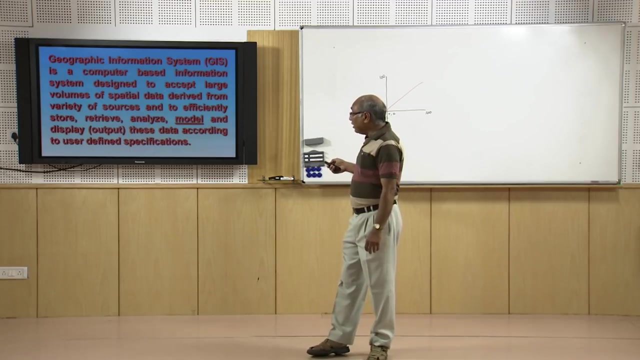 day which we are having, So computer based. it has to be computer based and it is designed to accept large volumes of spatial data, Spatial or geographic data. I have already explained to you that the data which is location specific data and which is designed to accept large volumes, that means a large data sets. 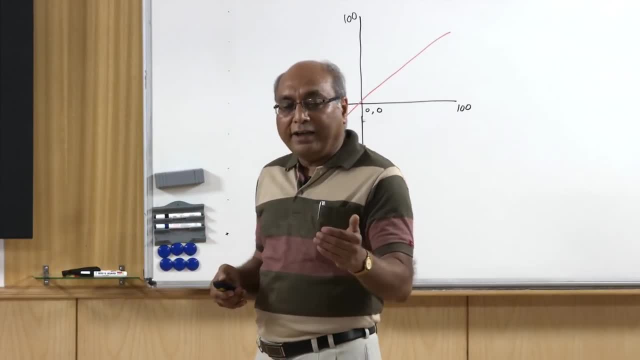 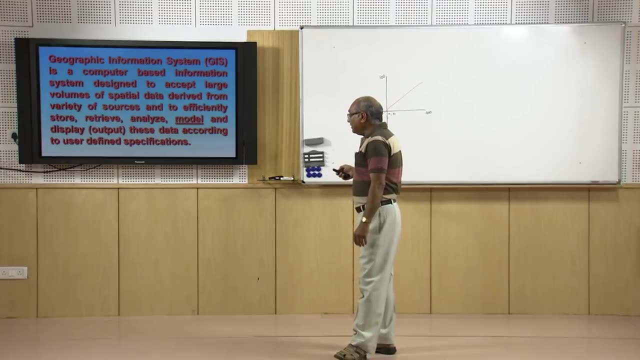 can come into our GIS database and then we can analyze in a very easily manner, and throughout this course we will learn how the analysis can also be found So computer based. it has to be computer based and it is designed to accept large volumes of spatial data. 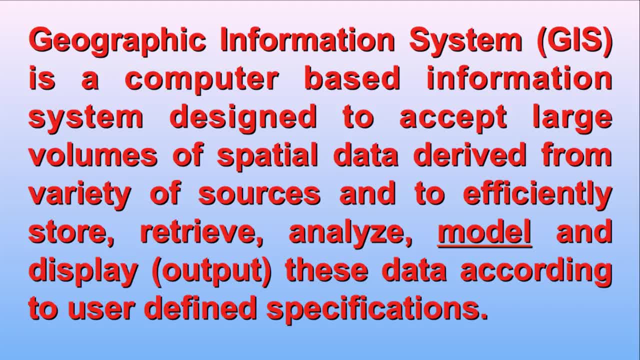 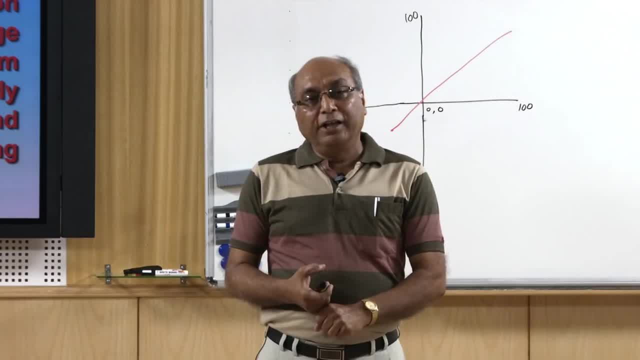 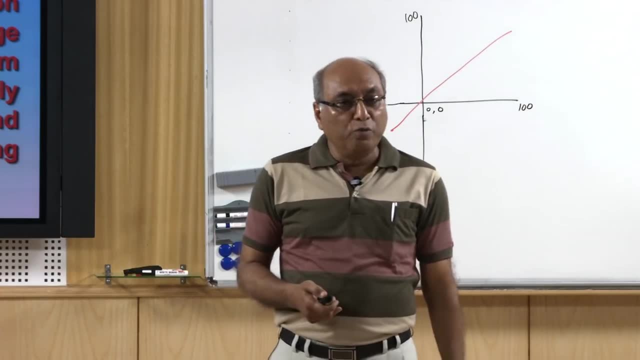 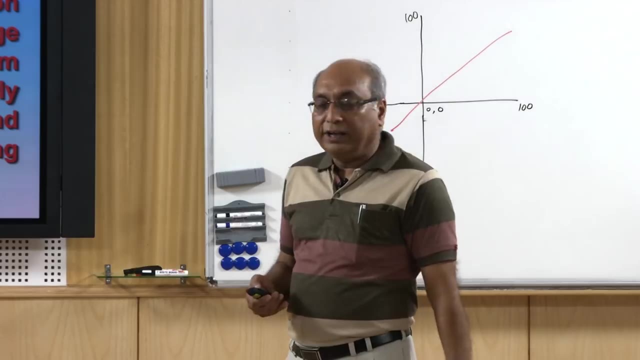 This data can come from a variety of sources. So these data are derived from variety of sources, Maybe the data, maybe the remote sensing data coming from satellite remote sensing, maybe data from field, maybe data coming from internet sources or various instruments. the data can directly come into GIS, given that it fits in the format which is required in a GIS database. 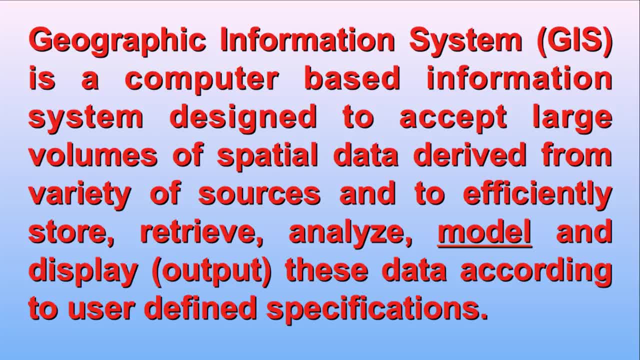 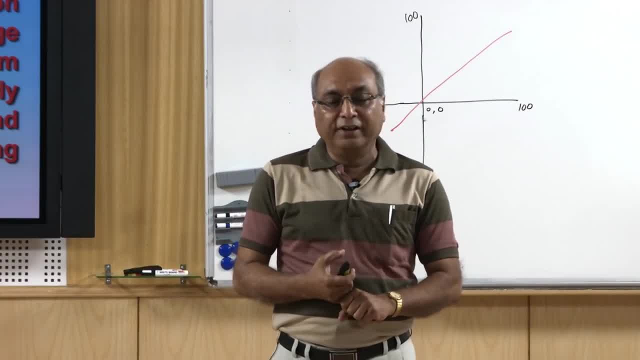 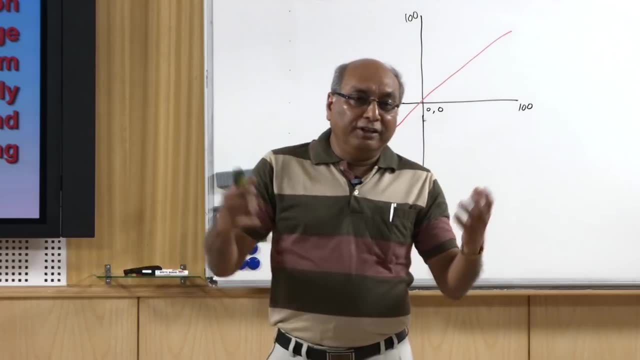 purpose of GIS is to efficiently store. if data is not stored properly, in a organized fashion, in a formatted fashion, then the retrieval of the data really becomes very, very difficult. for example, if a in a say, in a office, there are a room or a store which is having hundreds. 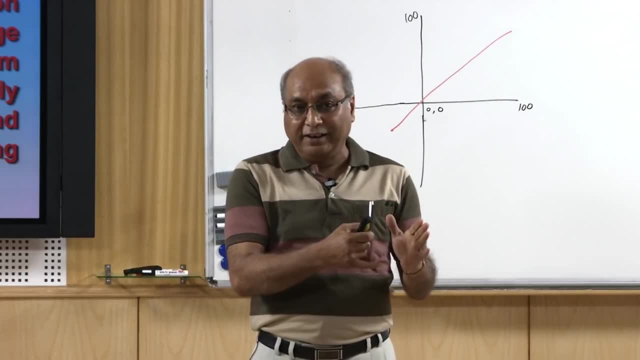 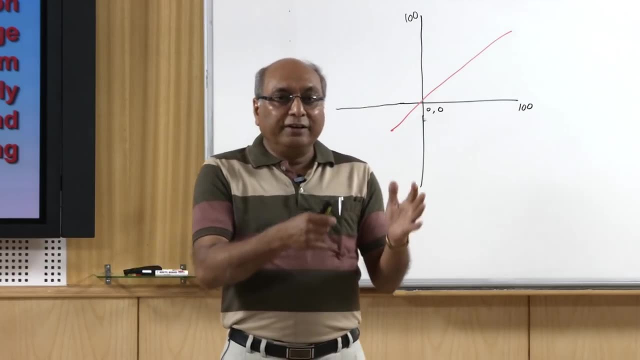 of files. we know that the information is there or data is there, but when I ask a specific data or information from that office, then the answer may come: sir, the data is inside the room or inside in this store room, but we do not know in which file the data is. that. 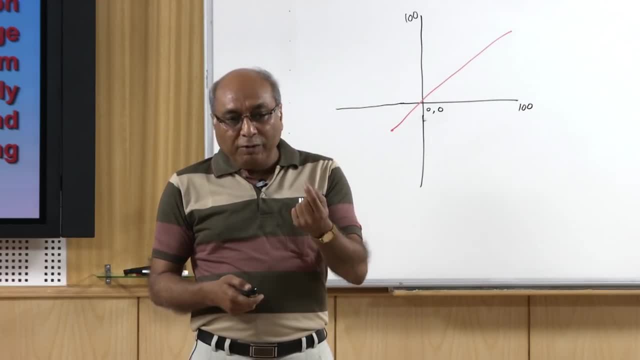 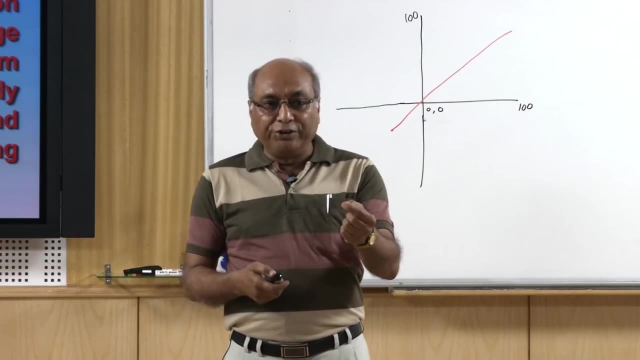 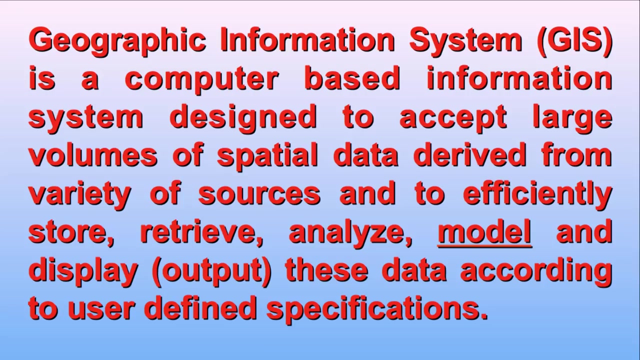 means it is not efficiently stored. if I am even, whenever I ask a question or data or information from that particular office and if they are able to retrieve very efficiently that information to me, then we call as efficient. so in GIS we can have efficient storage once we have a data storage. 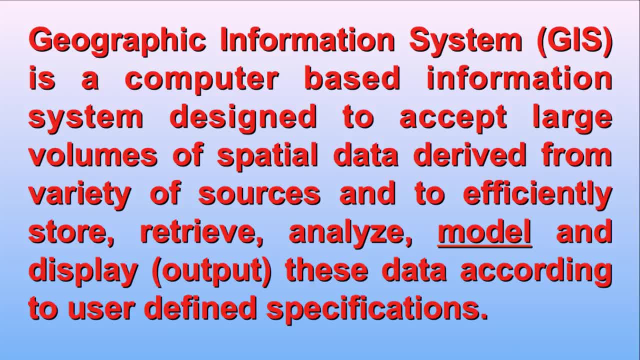 We are having efficient storage that allows us to efficient retrieval. and, of course, analyze, which is the heart of GIS. the main purpose of GIS is in these two terms: analyze and model model. I have given one example of ultimate aim of the model is to predict something which 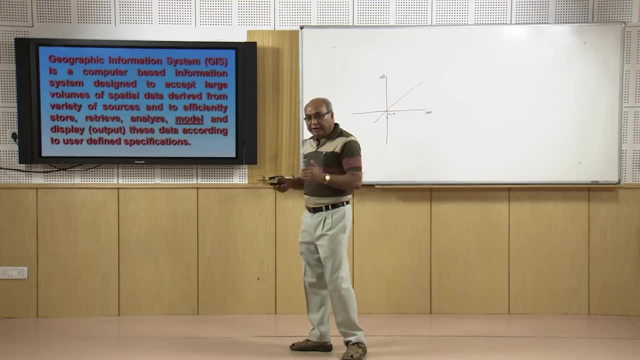 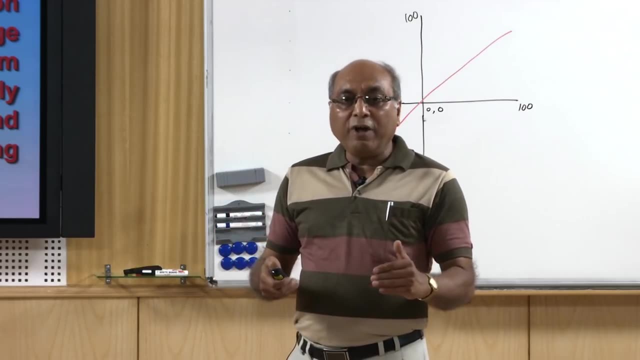 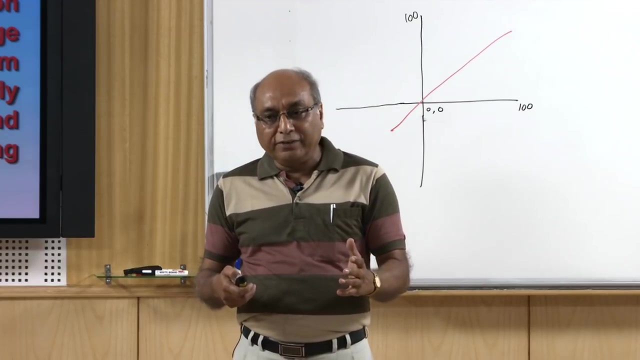 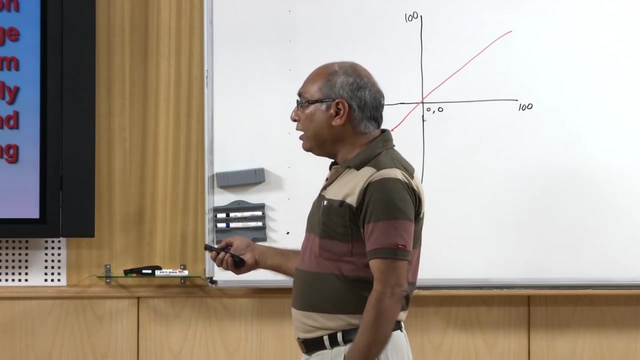 has not really happened on the ground. we will also see a demo in which a through a GIS software, I will show that, how, on a terrain, a reservoir can be simulated Before really it happens and we can calculate all, all required parameters which are required for the construction or even planning phases, pre-facility stage, so the model can be done. 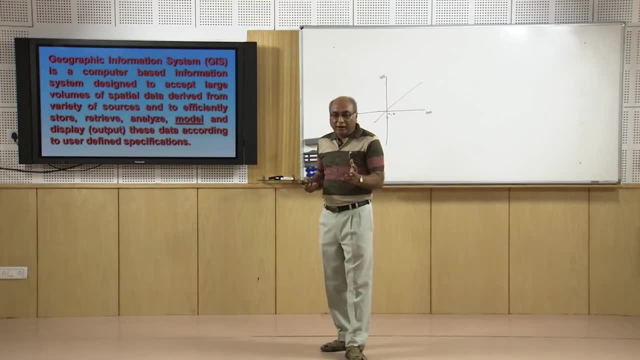 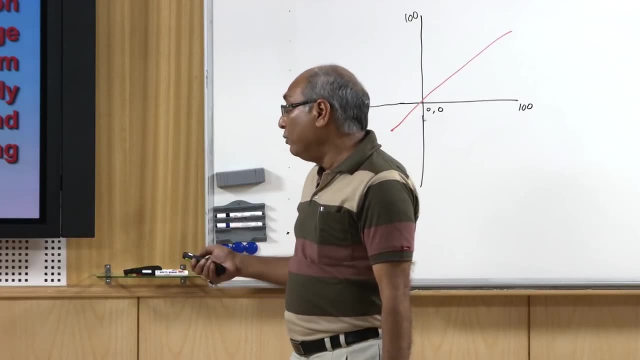 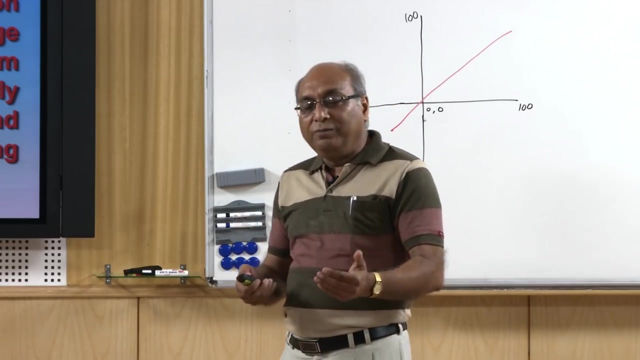 and various. then once you are having everything on computer, then you can play with that or you can change the scenario. you can change the constraints and conditions and can bring a very good you know, options or scenarios which you can present to the decision maker. So ultimate aim of GIS is to predict something which has not really happened on the ground. 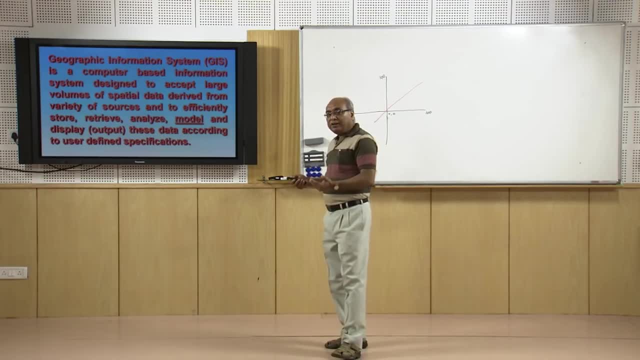 so it is a decision support system. So it will provide different scenarios through the analysis, through the modeling, which you can present to the decision makers and then they can make the appropriate decision. and finally, the main other purpose of GIS: to display or bring output. it is not just keep the everything. 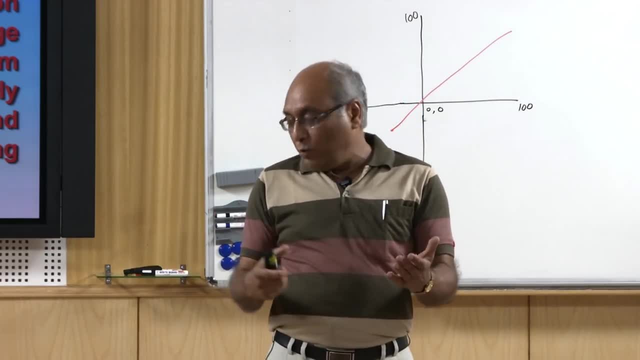 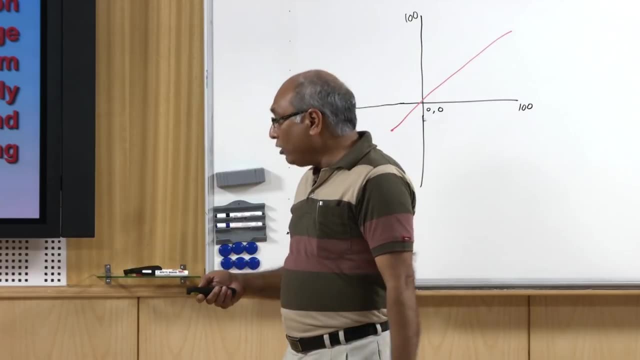 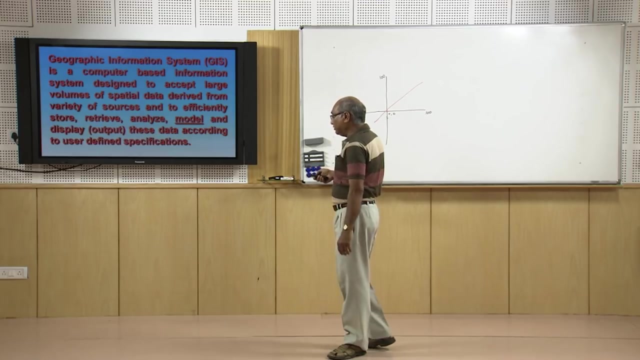 on the computer. no, you can create output in form of maps, you can create output in form of models, You can create 3D models and so on, so forth, or even simulations, animations. So all these things can be done at the end of the, you know, development stage of GIS. according. 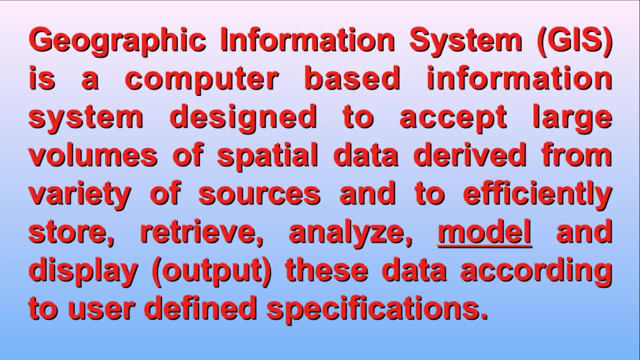 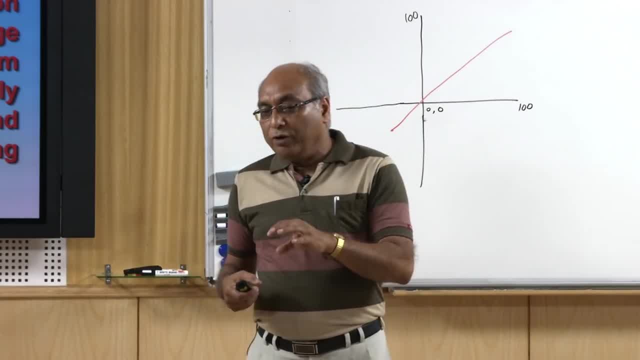 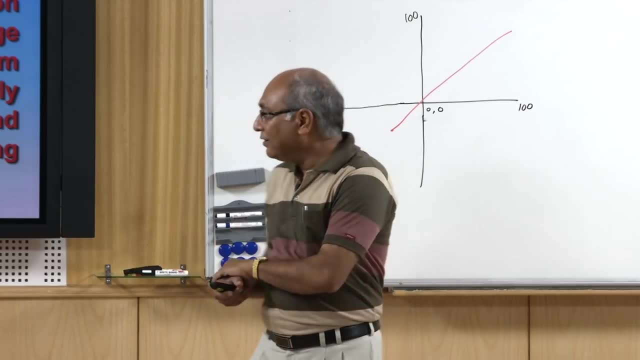 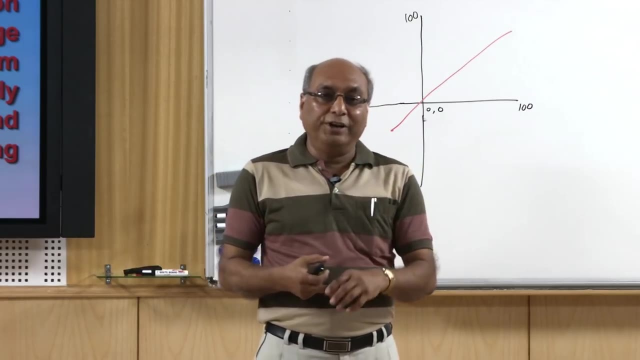 to user defined specifications. this is another very, very important thing, not as per the GIS expert, but as per the persons who is going to use the GIS data or output. So decision makers will ask something- this is very interesting- related to the development of GIS. Related with GIS is: more you deliver through GIS, more you are asked to deliver, and this 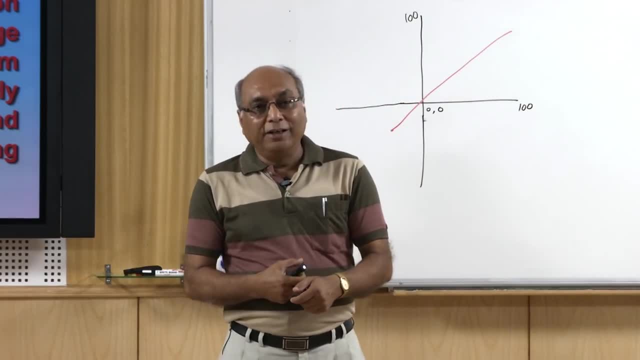 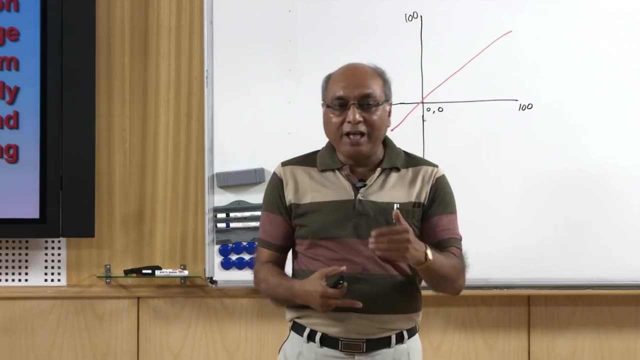 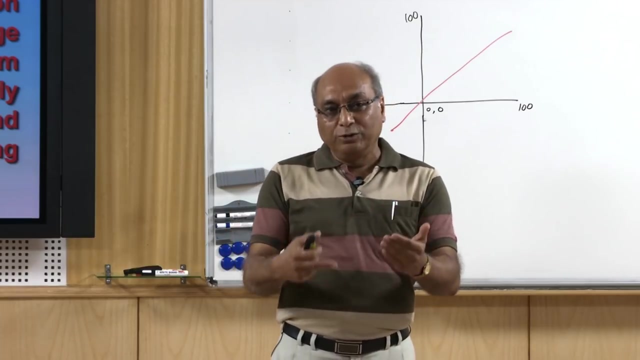 thing has really compelled us to develop GIS more and more, and this is how the Roger Tomlinson developed, because he was asked to do something using computers Once he developed the GIS. then he was asked few more things to do in the and slowly, slowly, this GIS has been developed. 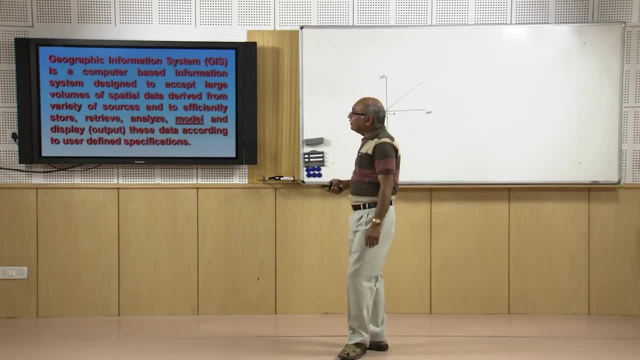 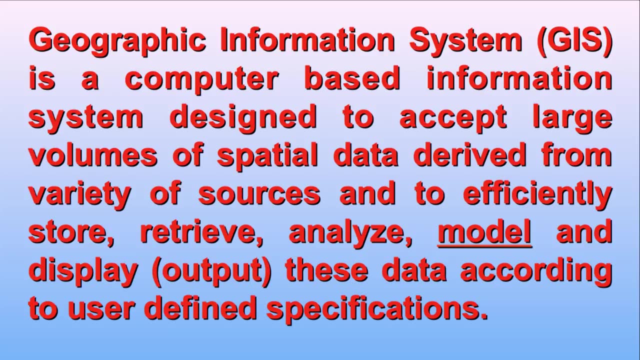 So let us conclude. So let us go through one quickly through. this definition is: the geographic GIS is a geographic information system, which is a computer based information system designed to accept large volumes of spatial data and derived from variety of sources, and to efficiently store, retrieve, analyze, model and display these data according to user defined specifications. 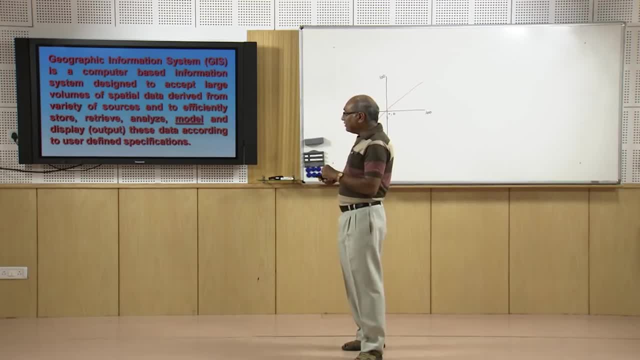 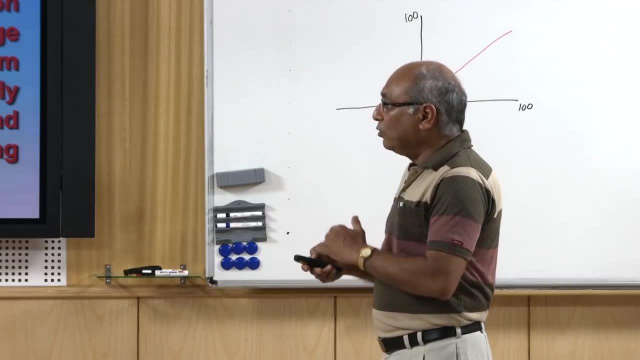 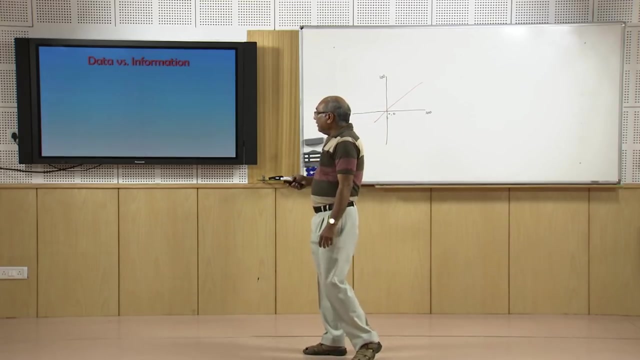 So users are very, very important. later on in the next lecture we will be seeing the different components of GIS where you will see the user or people are very, very important. So not only computer software, but the users are equally important in a GIS system. Now, I have been using these, these two terms generally, many people uses these two terms. 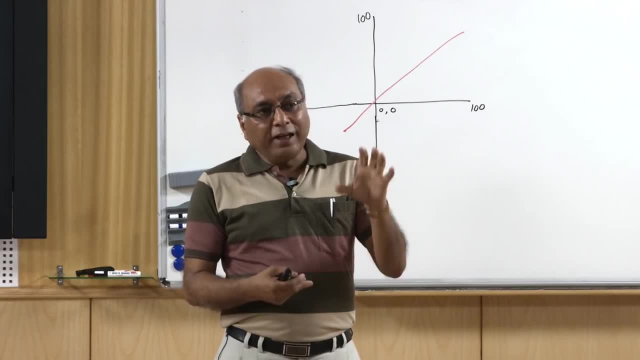 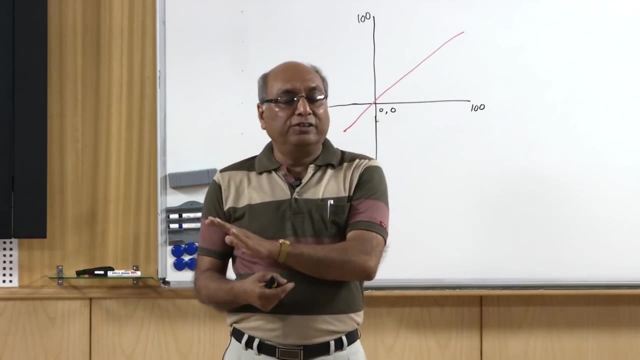 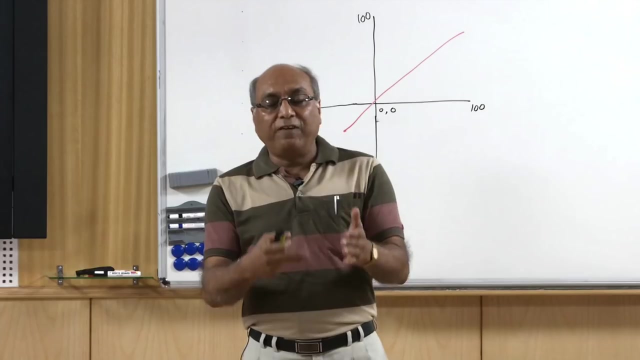 interchangeably, which is not really accurate. Data is something, information is something. and then, third, which GIS plays major, important role. So we have to convert all this into knowledge. So far we know that by data itself means if, if there is a register or a file which is 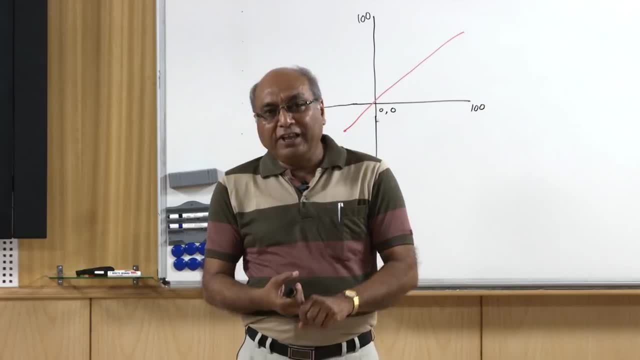 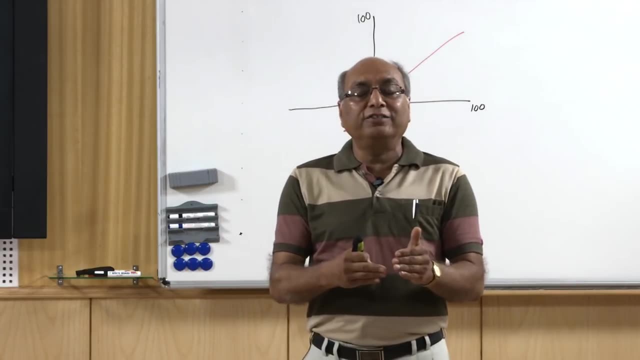 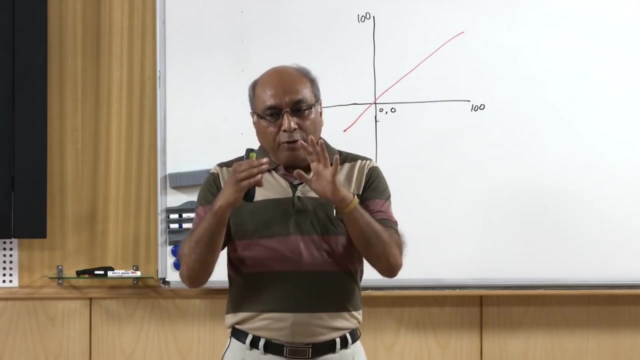 having just data, it does not have any meaning. Say, it is having a rainfall data, it does not have meaning unless it is analyzed. and once you do the analysis, perform analysis on GIS platform- then it becomes information. So using simple computer, even without using GIS, you can convert data into information. 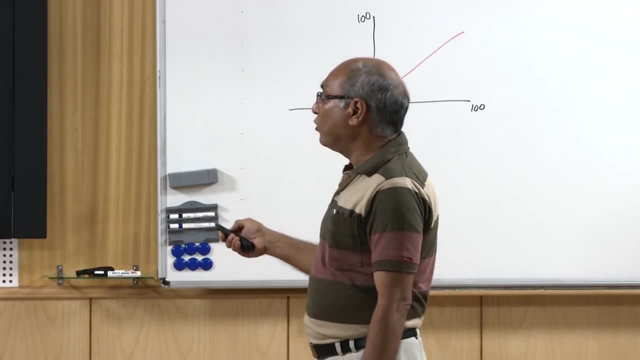 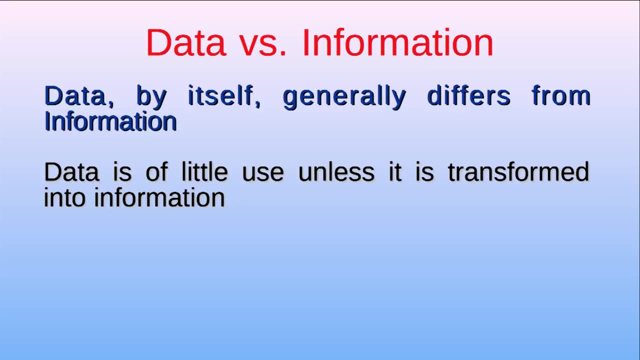 So data itself is a data, So data itself is a data. Data itself generally differs from information and data of little use, as I have already mentioned that if it is there in the file or in excel sheet or in a table or in a register, it does. 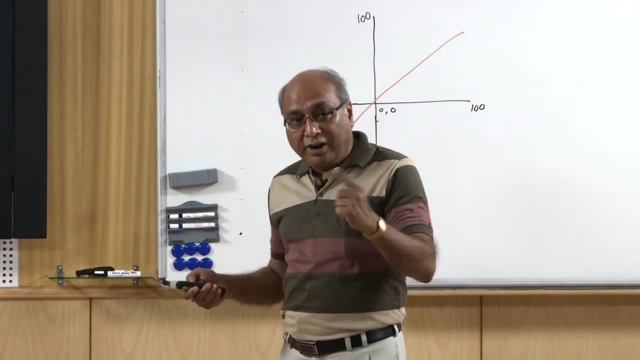 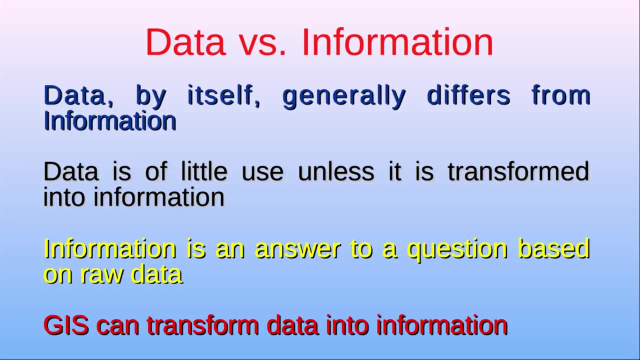 not have any meaning unless it has been analyzed and converted, transformed into information. The best thing which GIS does is even convert this information into knowledge, and I will give you some examples also. So information- Information is an answer to the question based on the raw data, whereas GIS can transform. 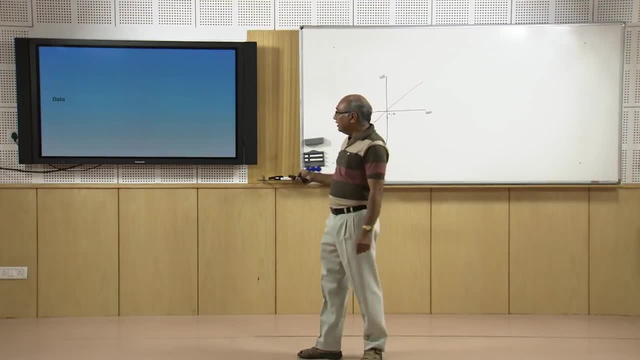 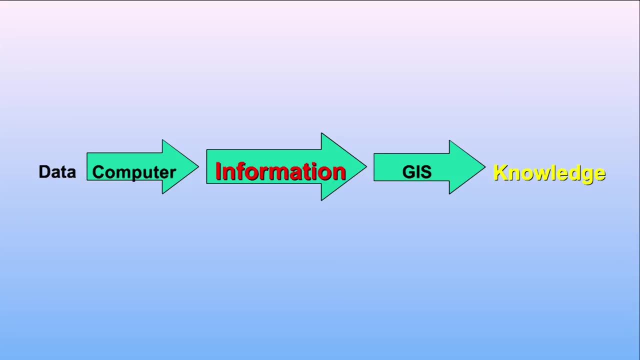 data into information. So how it happens, very simply, through a small fellow chart is the data. once you move the computers, you can convert data into information. But when this information goes through the GIS, then it becomes the knowledge. We have seen one watershed scenario where the forest was not yet cut, but we knew that. 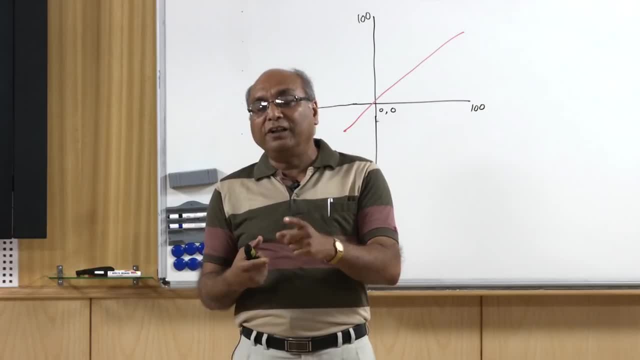 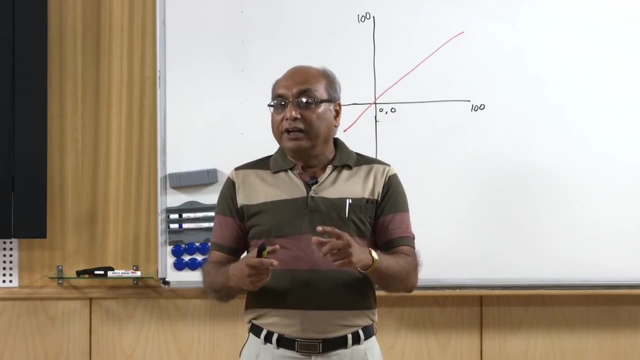 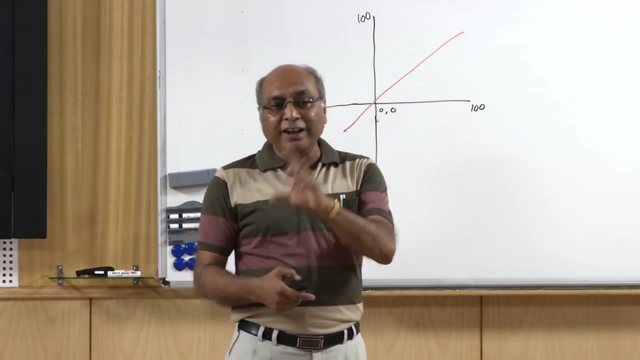 what would happen, What would happen to soil moisture condition, and that is the knowledge. So if, if GIS would not have been there, then such scenarios cannot be prepared or presented. and that is the advantage having GIS: that GIS not only converts data into information, because it is a computer based. 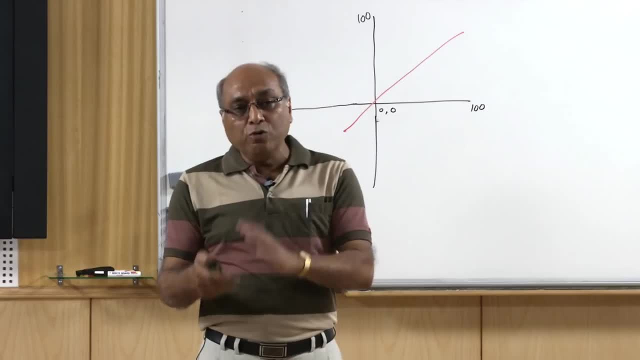 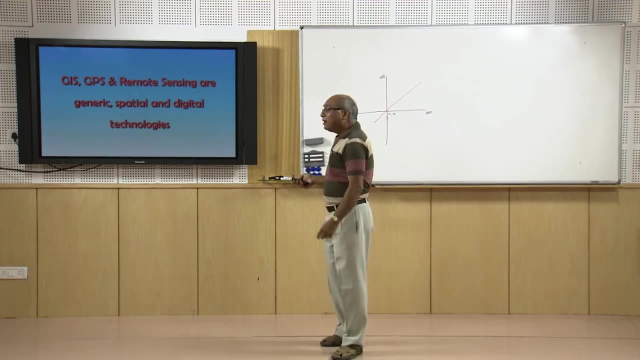 So it can convert data into information. but information, too, can be converted through modeling, through analysis in GIS, into knowledge, which is very, very important, And that is the best thing. So that is the knowledge, So that is the basically what I would say. the ultimate purpose of GIS is to convert data. 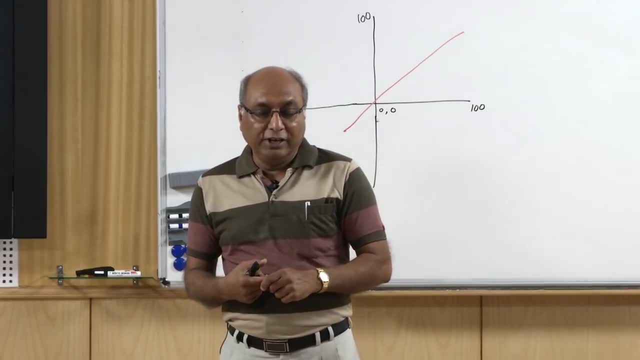 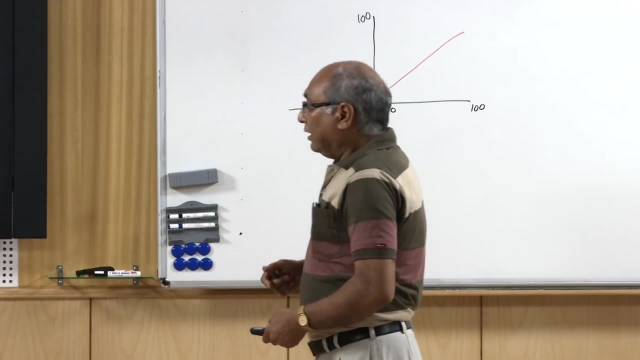 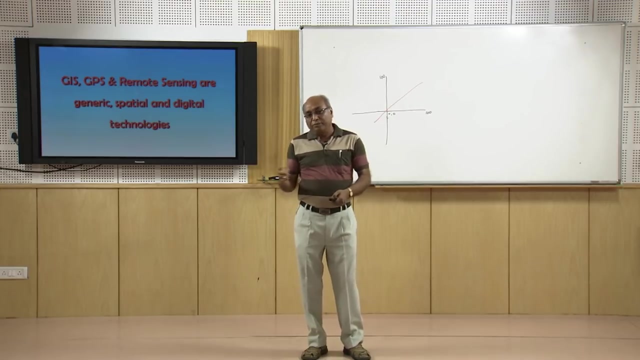 into information and then, finally, to the knowledge, and knowledge which can really help in all kinds of scenarios, which we will see little later Now. I have also mentioned two other technologies. One is GPS, another one is remote sensing and GIS. we are, we are already discussing here. 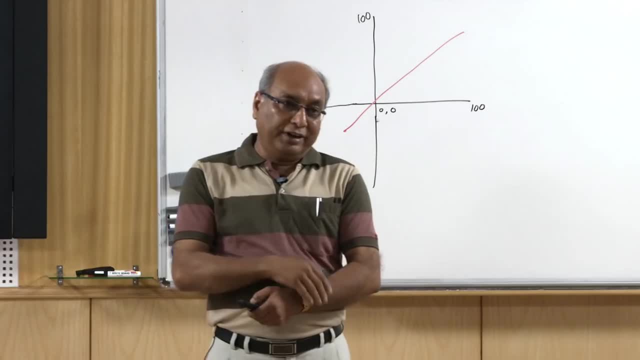 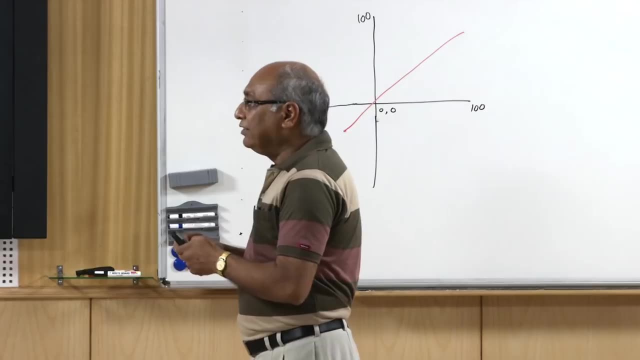 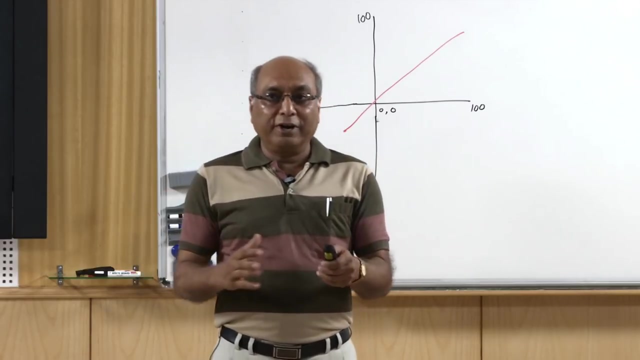 that. But there are three common things with these three technologies, very, very important, and that is why, because of this, these commonalities among these three technologies, the the integration of these technologies have become very much possible and therefore new, new product, new new applications are coming through this, which we will see some examples. 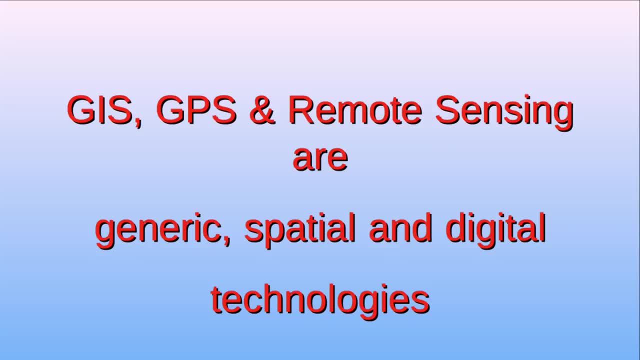 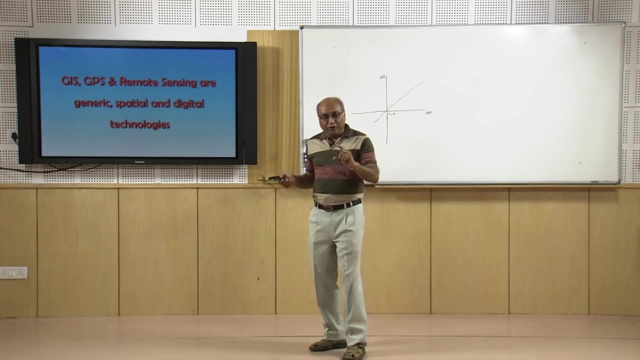 So GIS, GPS and remote sensing, which is satellite based remote sensing I am talking, are generic. I will explain. I will explain. I will explain spatial and digital technologies as a spatial or geographic technology, which we have already said, that, because GIS handles the data in geographic domain, GPS provides 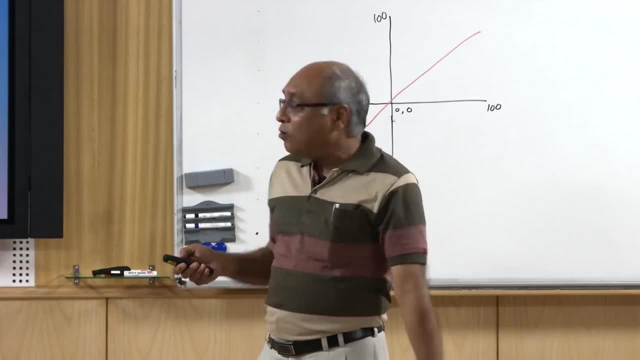 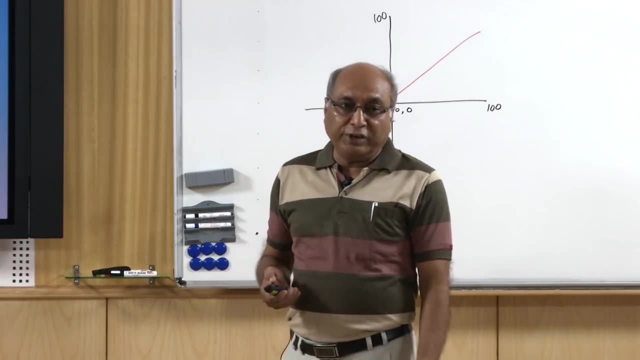 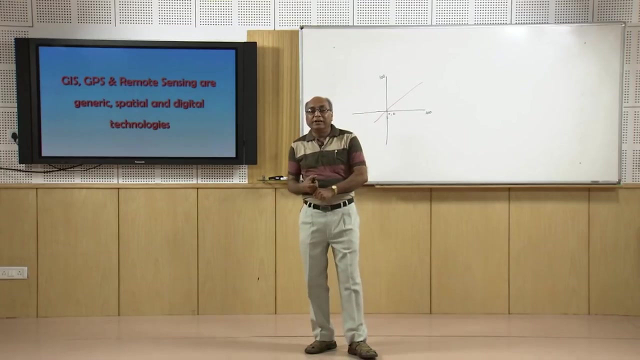 the geographic coordinates on any part of the globe, anytime, and then remote sensing data is also represented in, can be represented in a spatial domain or in geographic domain. Now now about the word generic. Generic means here. Generic means here that it can be applied for various things like computers, you know. 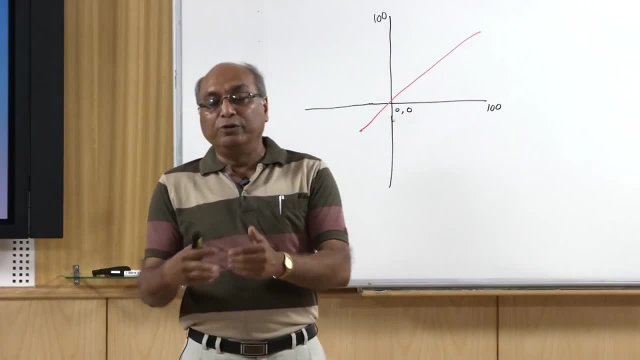 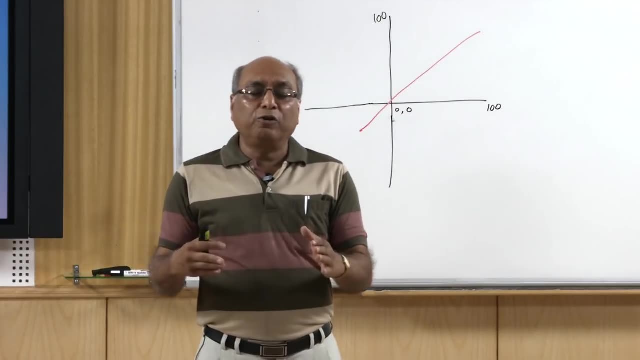 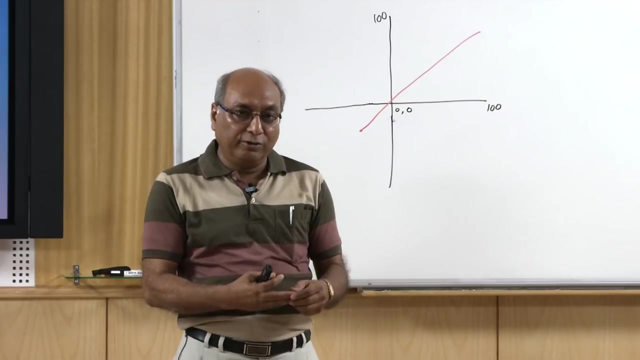 computer are being used for accounting, computer are being used for creating videos, computer are being used to modify, you know, audios all kinds for all kinds of purposes. nowadays people are employing computers, So computer technology is a generic technology. So our these three technologies, which are like GIS, GPS and remote sensing, 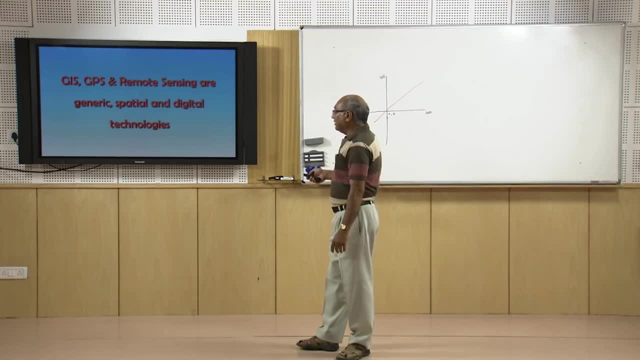 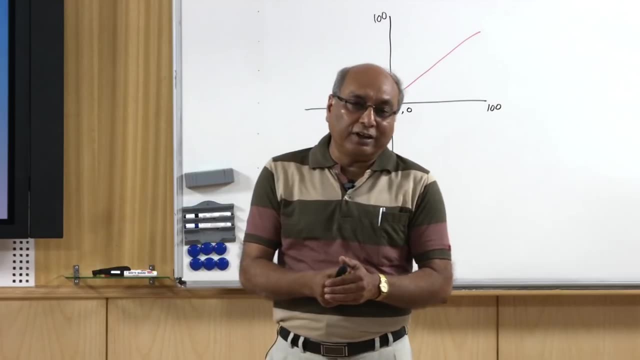 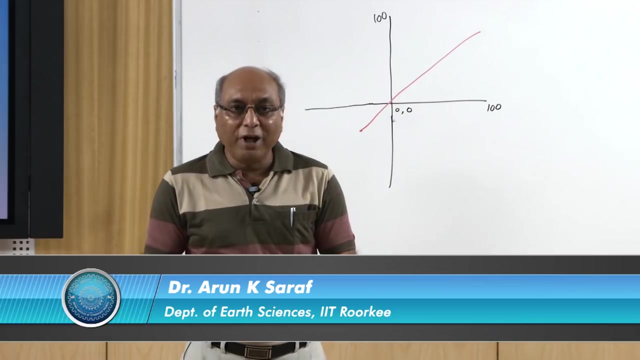 Are generic, Spatial And digital technology. Since these are digital technologies, therefore, the integration of these three technologies built computer technology has become very much possible and, as we are seeing nowadays on your mobiles, smart mobiles, all kinds of things are coming and one of the two best 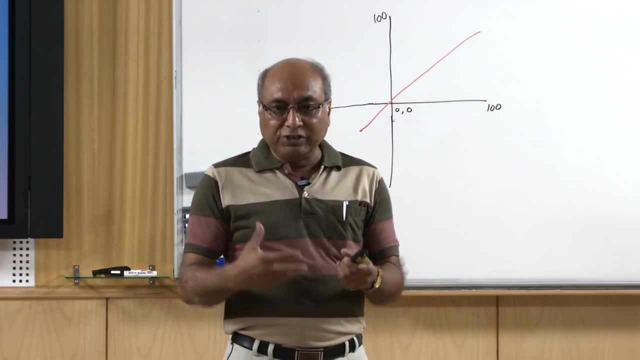 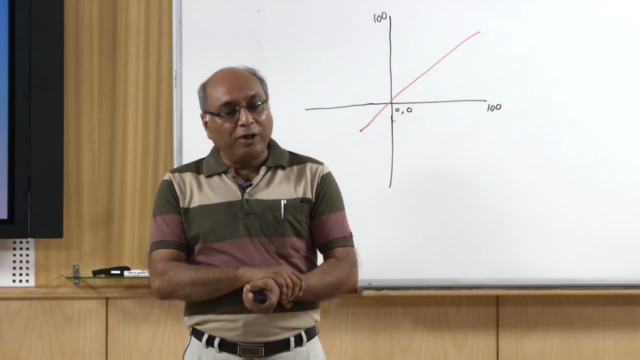 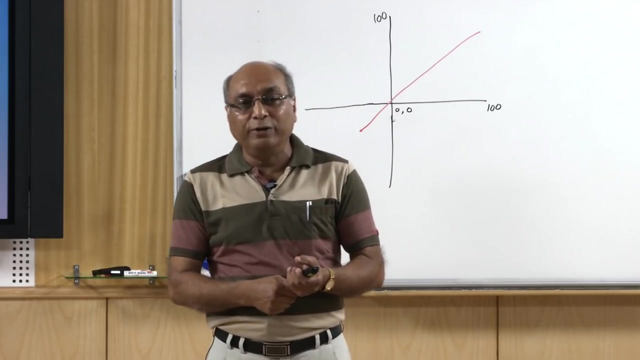 products which people, unknowingly, which which are not expert of GIS, they do not know what is basically GIS, May not be knowing, But they are using these very popular products which I can name. one is Google map, which, on your mobile, anywhere you go, for navigations, for car navigations, location identification. 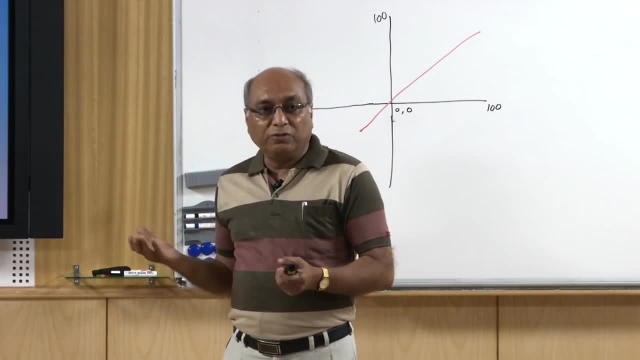 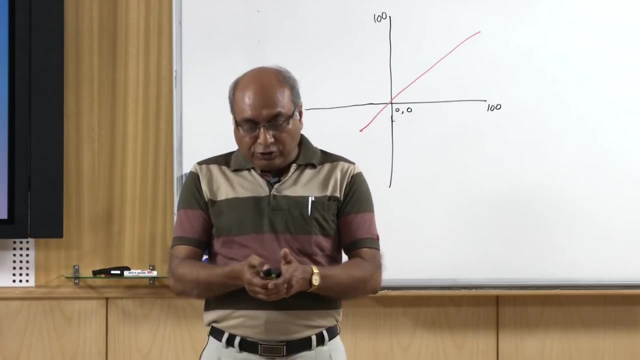 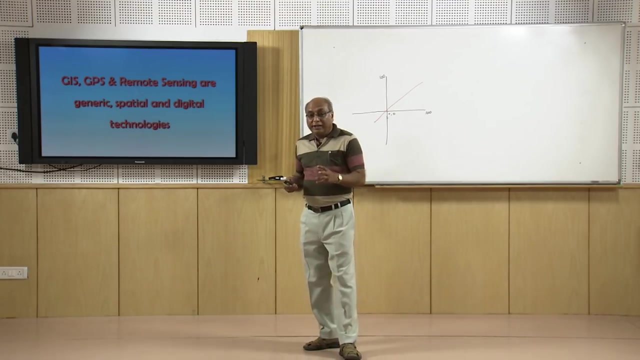 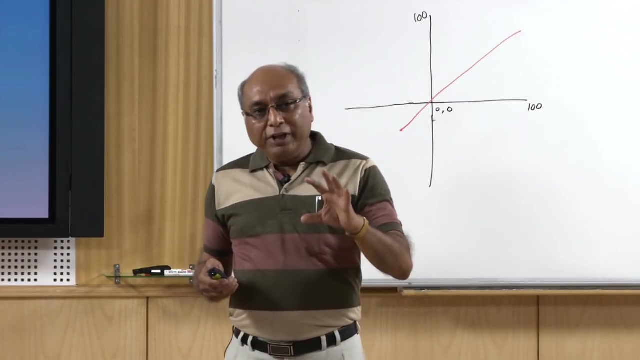 for all kinds of things. you are using Google maps. So Google map and Google earth are the custom design very spatial products which uses all these three technologies in integrated fashion, And this is how The growth of A GIS and and on these technologies is reaching to the common man without even they do not. 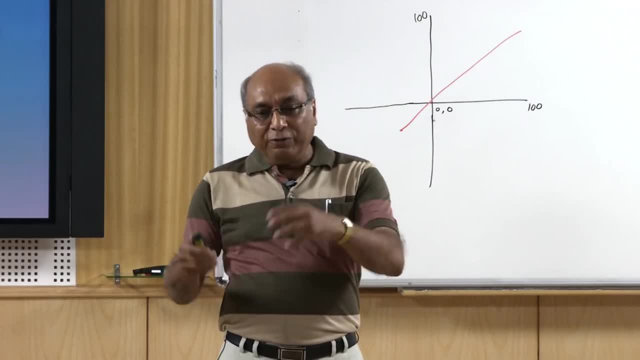 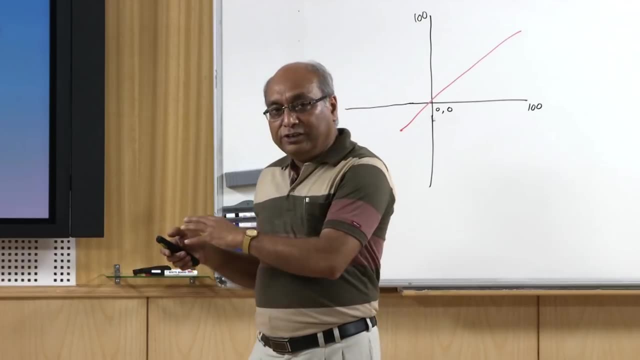 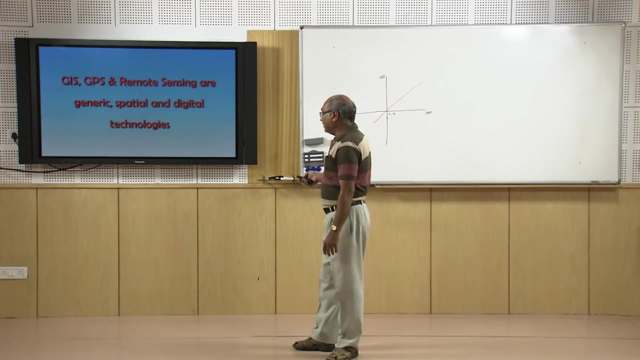 they know, they do not know, they are not aware that what kind of integration of technologies which they are using, even on their mobiles, But these technologies are being reaching, are are reaching to the very common man through such technologies like smart mobiles and other things. 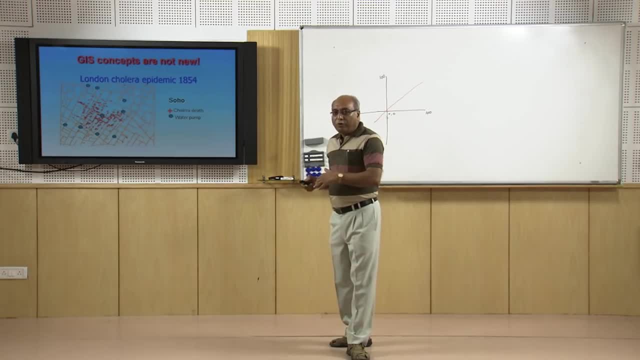 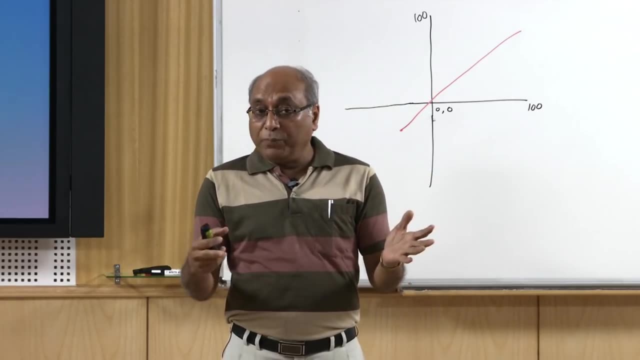 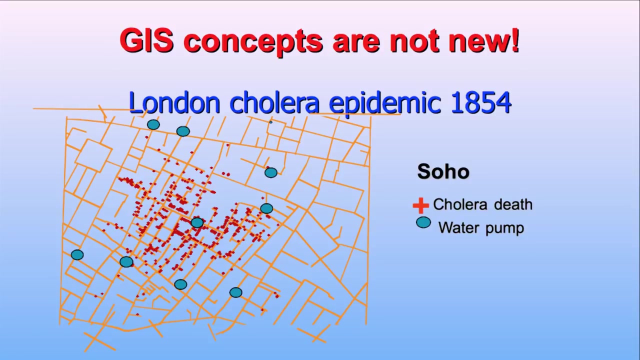 Now, As I have mentioned, That Even before Roger Tomlinson the concept of GIS in analog form was already existing, But not the present GIS, and I had lot of limitation nonetheless, there is one example of 1854 in London. they were cholera epidemic, and what people analyze that? there are some ah water. 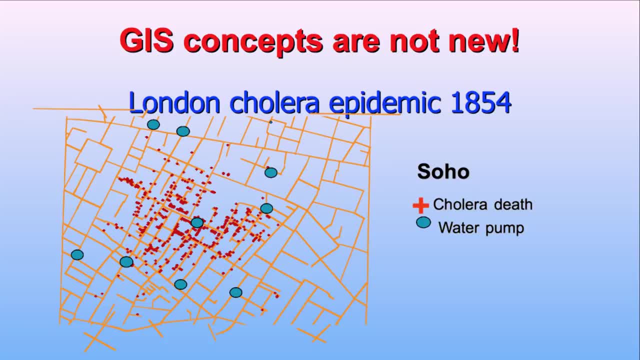 supplying tube wells and there were deaths due to the cholera and when this plotted, when this deaths were plotted, using geographic coordinates On a road map and having this location of a water supplying tube wells, they found that the not all wells water is polluted or having problems, which is causing cholera. 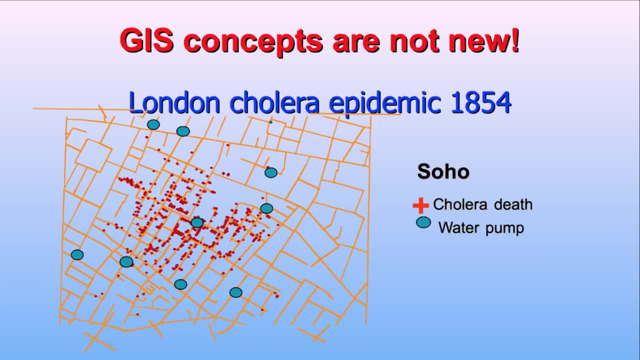 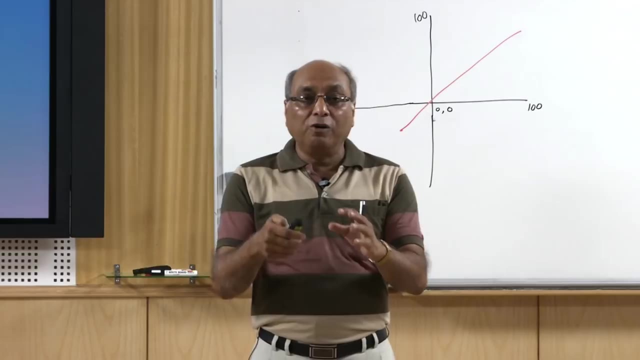 Only few wells, especially the well which is shown in this map in the center was the most responsible well which has the water which was causing cholera. So once as I gave the example of GE selection, Similarly Lot of such problems Can we resolve or can we? these challenges or problems can be understood once we start. 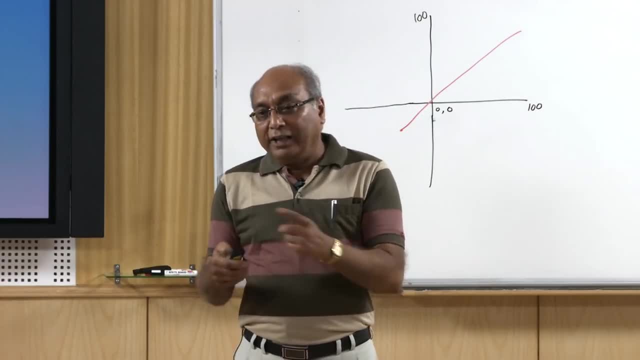 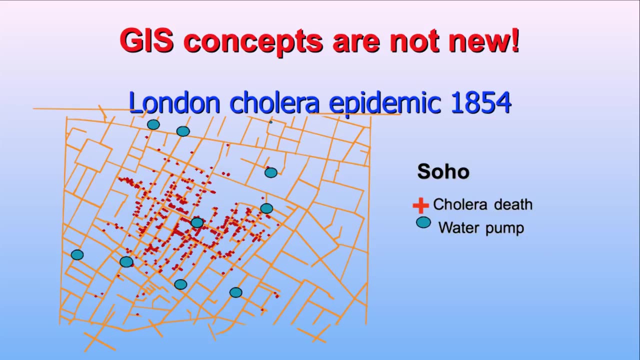 plotting the data using geographic coordinates and, as in this example, also. So once the data is plotted, immediately one can raise the question that why the deaths are due to cholera are surrounding this area. why not in other parts? and obvious answer: that might be because of. 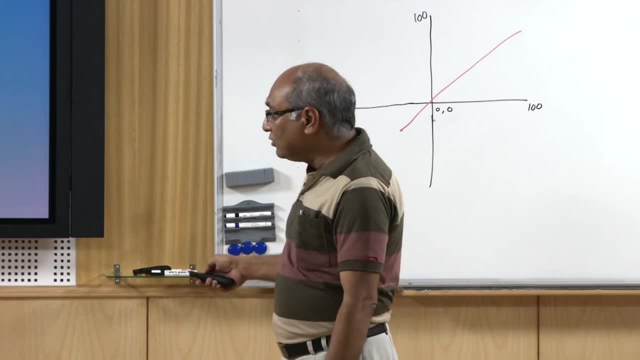 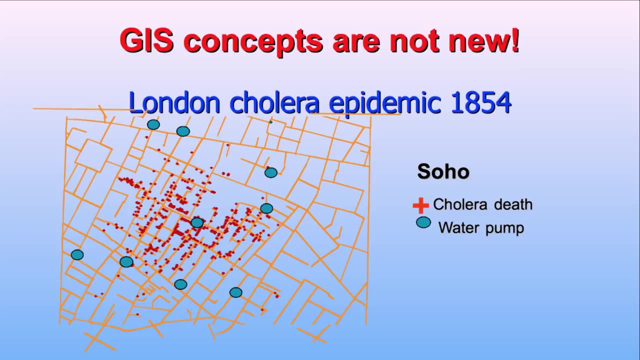 So One, one layer is not sufficient, as you are seeing here that the three layers of information, three themes, are there. one is your street map, another one deaths due to the cholera and third is the tube well locations. In GIS you can have several such layers. this is analog system example, but in digital systems. 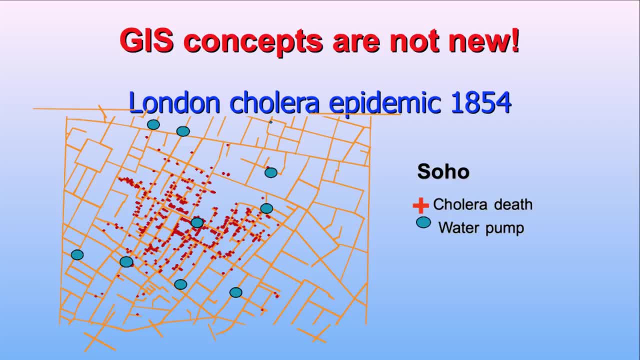 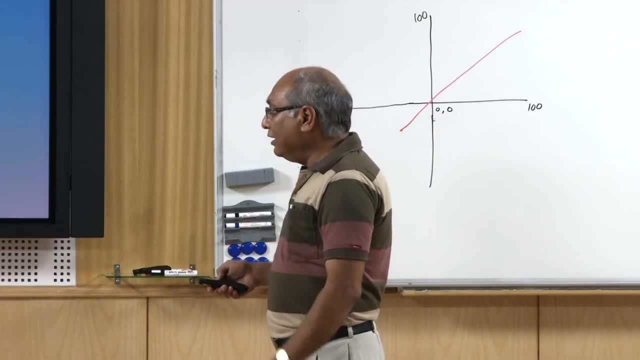 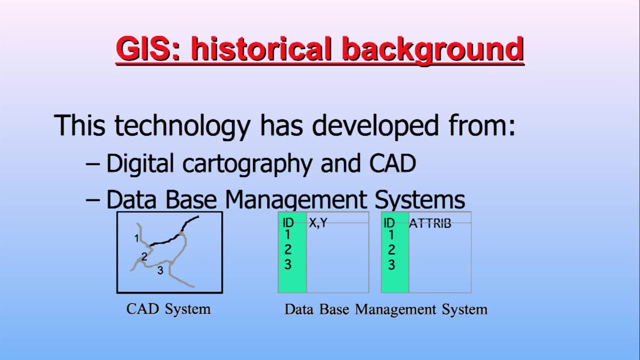 you can have variety of data, variety of spatial data, into GIS system, variety of layers of all kinds Which we will learn in this course slowly. also, it allows us to store the data in tabular form, which that means it is at this: spatial information is attached with attribute data. 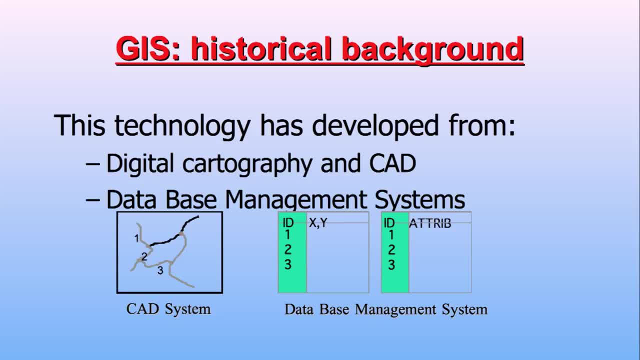 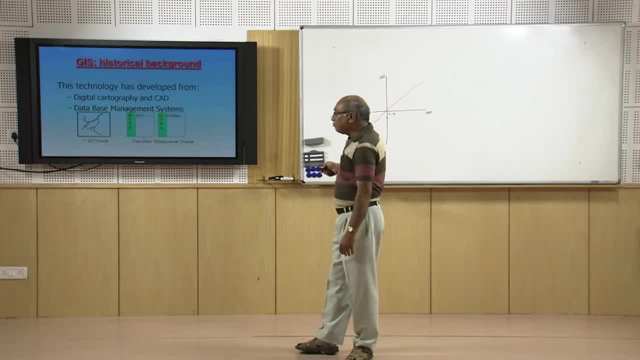 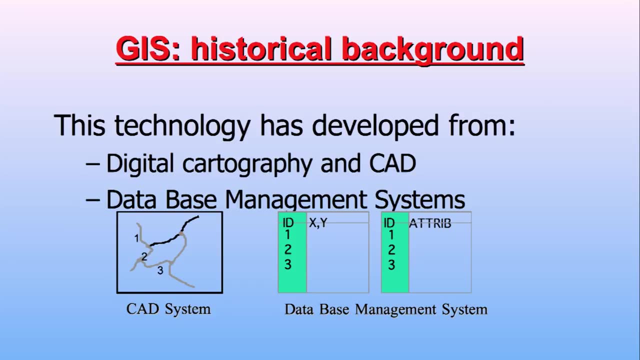 which we also call as non spatial data. as I have said that, the GIS is a integrated technology, So you are having digital cartography and CAD, CAM tools are all available in GIS, plus your database. So all these technologies have been integrated into GIS, plus few more things and the basic. 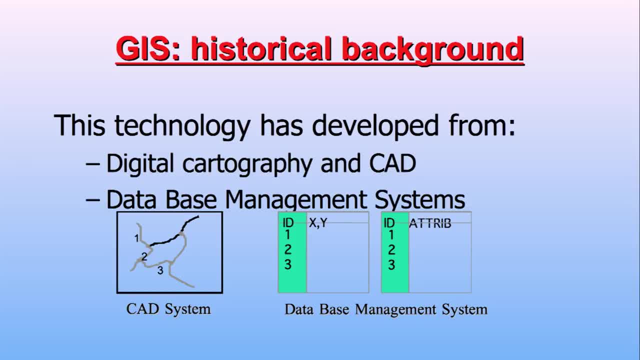 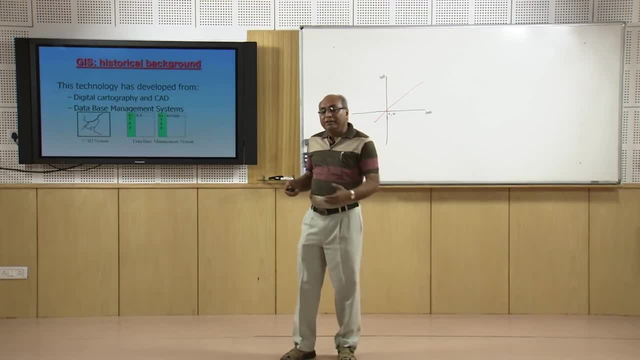 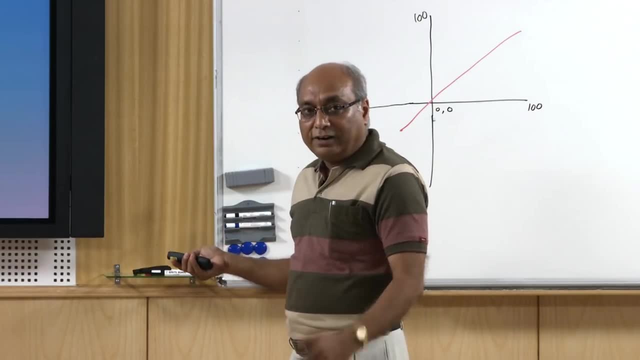 thing is handling of all this in geographic coordinate system. So in that way, analog GIS systems are not new, but only this digital GIS systems developed in somewhere in 1962-63 when Roger Tomlinson started developing GIS. as I have mentioned that a data in GIS is scalable. 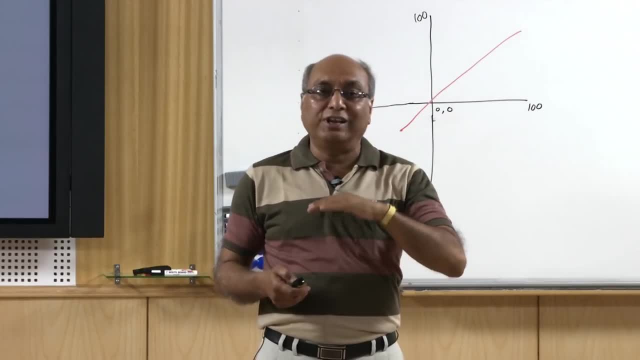 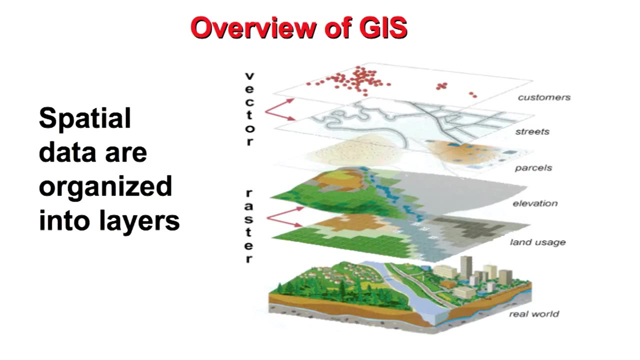 It is kept in different teams or we call, in simple terms, and layers. a real world example is given here, that this is real world, which is having, you know, natural features like streams, hills and forest, and some manmade features like buildings and roads and other things are there. 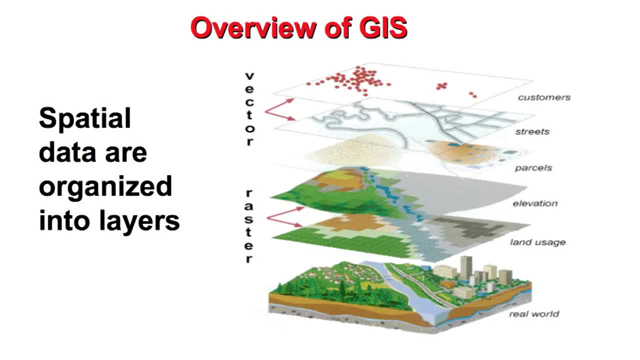 Three dimensional information is also shown here what we can do in GIS, that we can keep different information in different layers, Like here: the land uses, how the land is being used, can be kept in one layer, which when we can call as land use layer, Then how the topography is changing, that we can store in a elevation or in a raster layer. 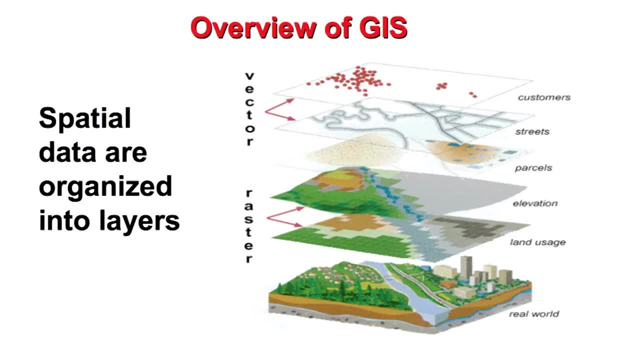 which we call as a digital elevation model, in elevation layer. Then how these land records, who owns which part of the land, revenue records, can be stored in a polygon layer, Which is here it is mentioned: parcels, So it is a polygon layer, and then you are having a road network or a street network. 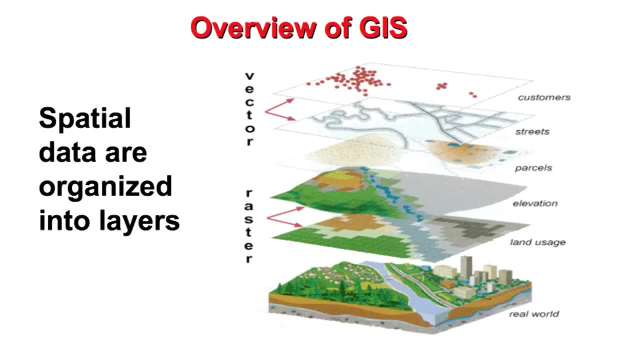 which you, which is nothing but the line network which you can have in another theme, which is a street network, And then you are having locations, maybe resident customers, patients, all kinds of things, as a point data. you are storing So all variety of data, as you can see that there are point data. 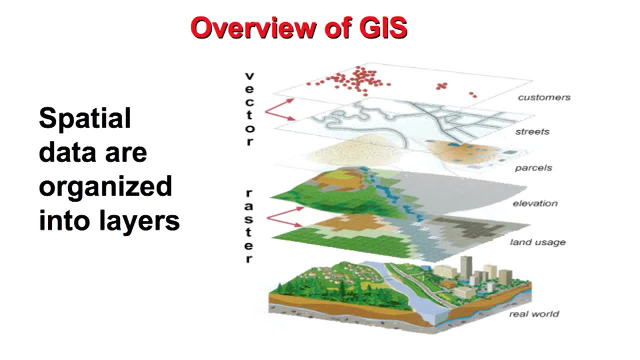 There is line data, There is a polygon data, and then these two data sets are different, which are a continuous data, which we call as raster data. So this is raster data, This is vector data. So vector- all three types of vector data- is there here. we have not added satellite image. 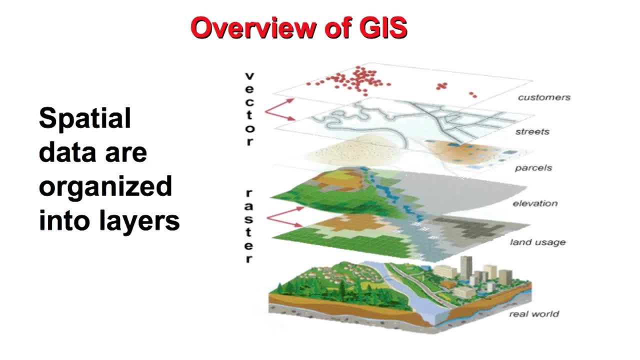 You can bring one more raster as a satellite image, that will go as a raster data. So what we see here, that the real world can be divided into several layers. Now, anytime, Anytime we want to use any of layer or combination of these layers into a GIS system. it is very 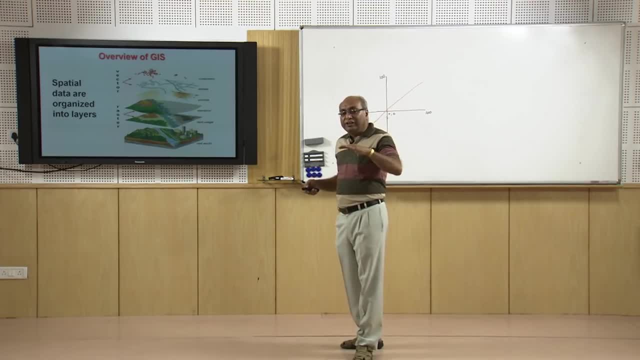 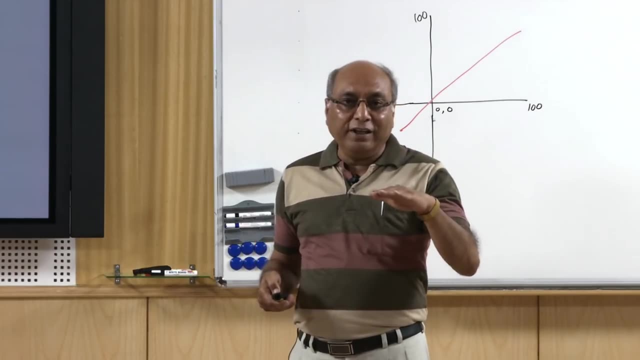 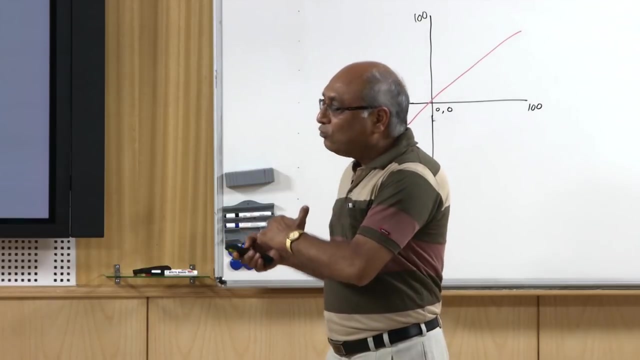 easy to use and that is why this this initially the at the data storage level. we go for this disintegrated manner. We store data in a different layers, different themes and later on, whichever the theme is required for my analysis, I I will use, Like in case of that cholera epidemic, three layers were used: the groundwater level data. 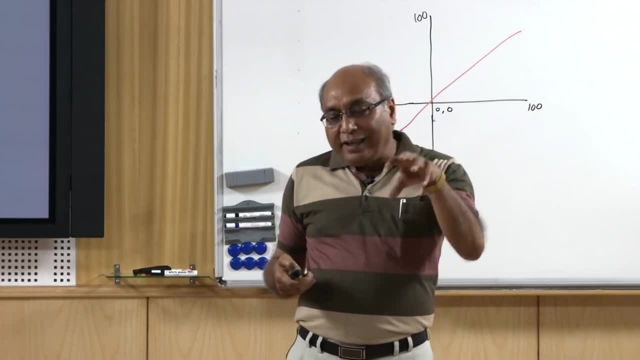 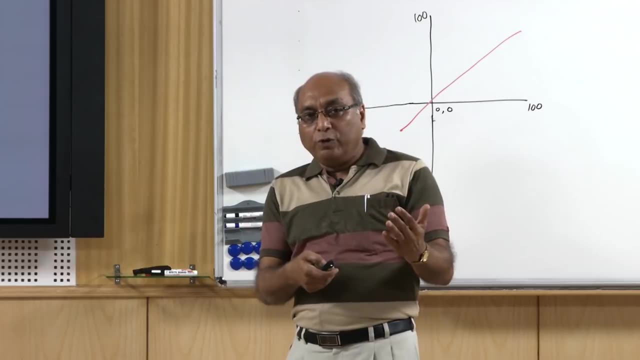 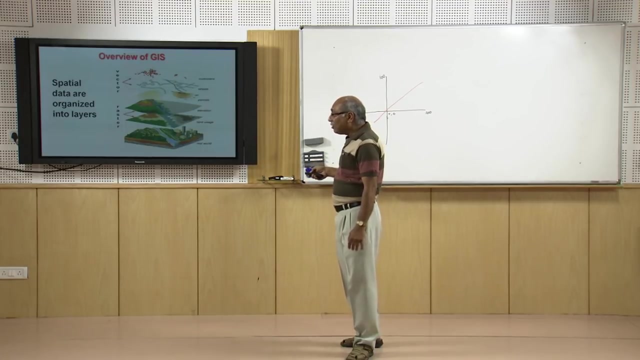 street level data, The water level data, The water level data And then deaths due to the cholera. So only three layers were used. depending on the problem or solutions which you are looking, you might use different layers. So basically, as you can say that in GIS, these layers are, the data is organized into- different 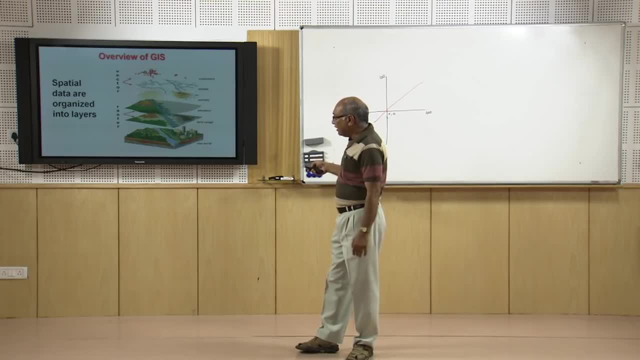 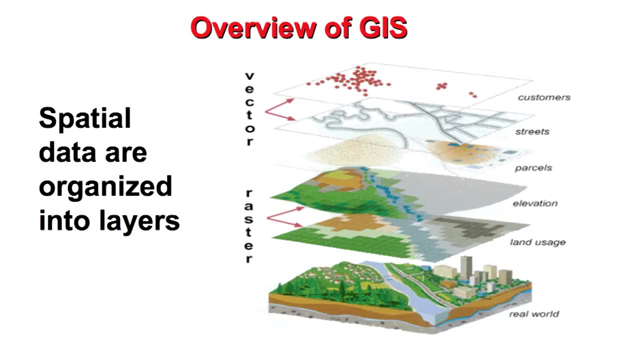 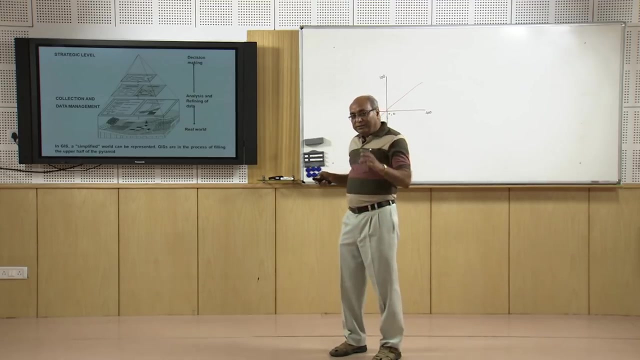 themes or layers, having two or three different types of data models. One is vector raster and one more data model, which we will be discussing in later lectures, is the TIN. This is triangulated irregular network. Now, as I have said that GIS ultimate aim is to support decision making and this is how. 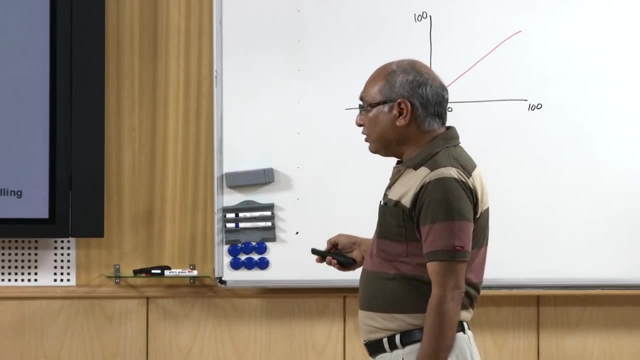 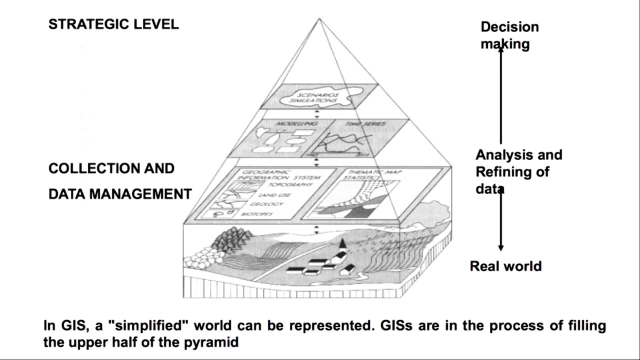 done at strategic level. So again the same scenario here, that a real world is a segmented into different layers and data is collected, then you create, through the modeling analysis, you create the different scenarios and then decisions are taken. Another very important thing is that these arrows are two directional. 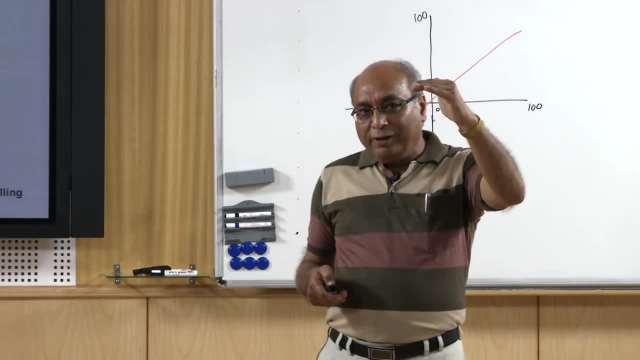 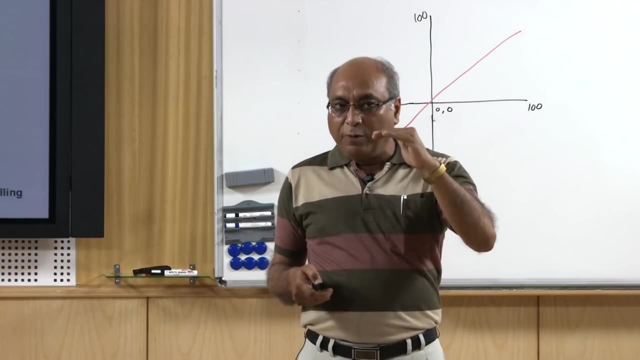 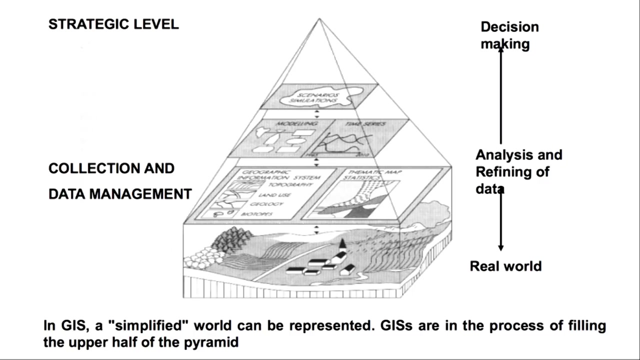 And that clearly indicates that at the decision level it may be decided more data is required or the answers which, at decision level, people we are looking are not getting, then we have to come back And that is why go back to the real world, collect few more data maybe we have to collect. 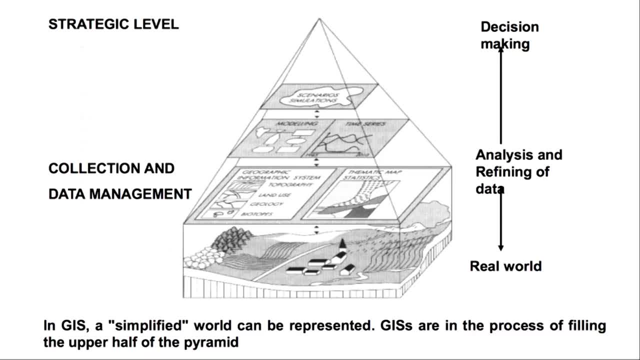 the subsurface data, like groundwater data, or maybe the soil type data, or maybe lithology. And that is why go back to the real world, collect few more data. Maybe we have to collect the subsurface data, like groundwater data, or maybe the soil type data, or maybe the soil type. 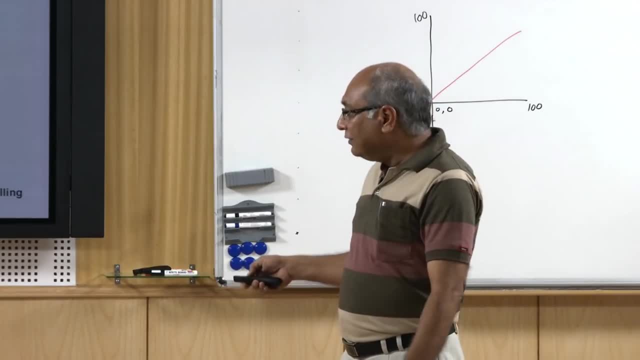 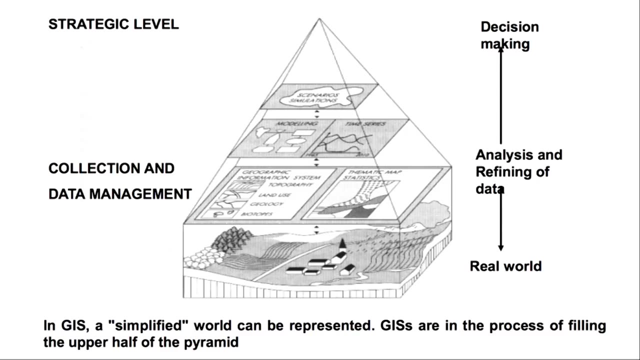 Or maybe if we are looking for groundwater exploration, then we have to go for subsurface, So we will come back if at this level the answers are not coming. we go back to the real world, collect few more data layers and then develop the scenario again. and when we are, 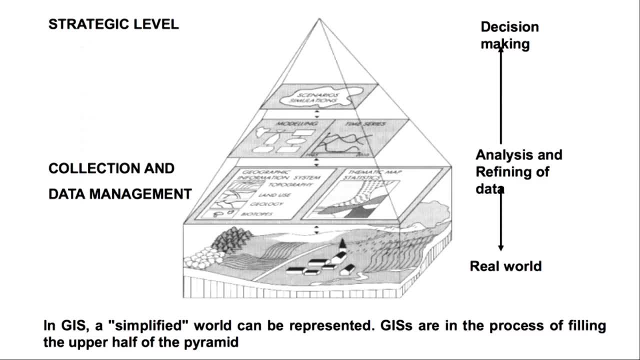 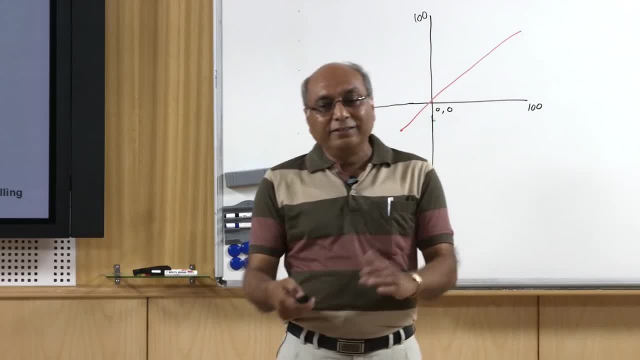 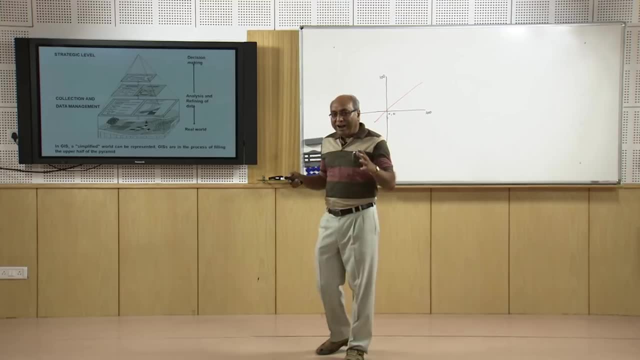 able to supply the data to the decision makers or the scenarios to the decision maker. GIS expert himself can be also decision maker. that the GIS expert cannot be decision maker, But in many times there are people- those who are- who do not know how to handle GIS. 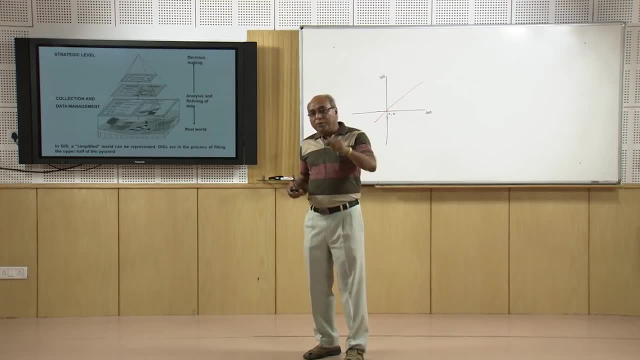 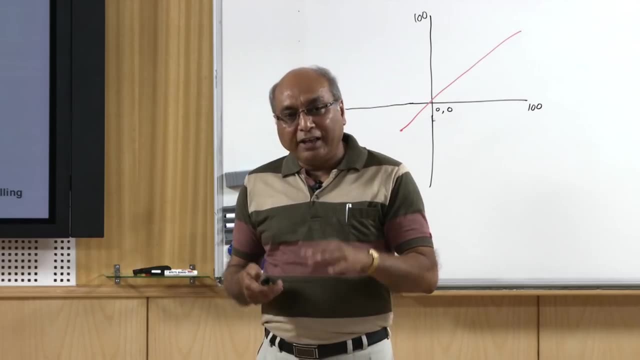 They do not know the concepts of GIS. But these are the people who keep raising questions about: can you do this thing, can it be done through the GIS, and so on, so forth. So, therefore, this is a two directional thing. Both directions it works. 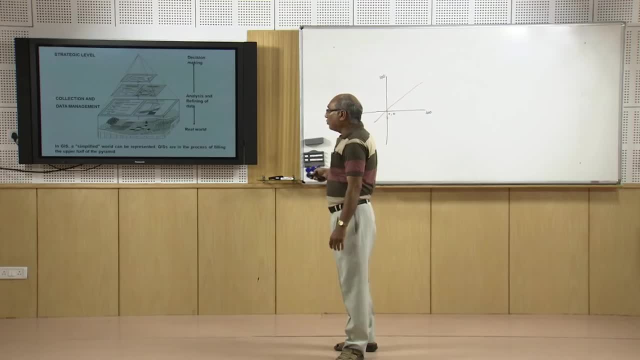 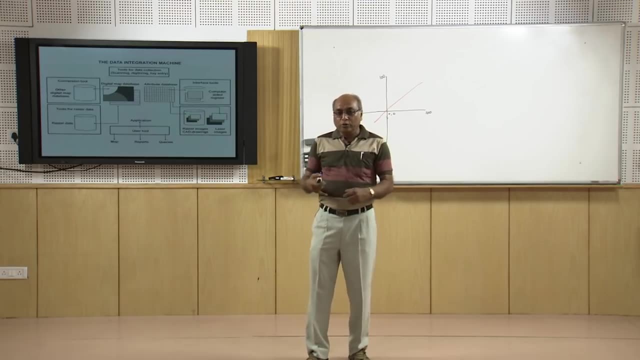 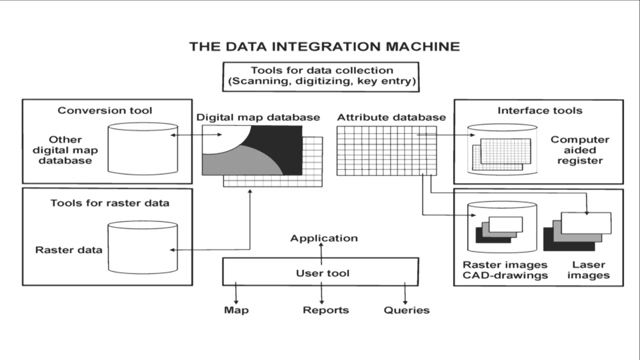 So it is a simplified version of the real world and the processes which are involved here. GIS is an integration machine, as indicated earlier, So you are having data from coming from variety of sources, that data you organize in a special domain, and so on, so forth. 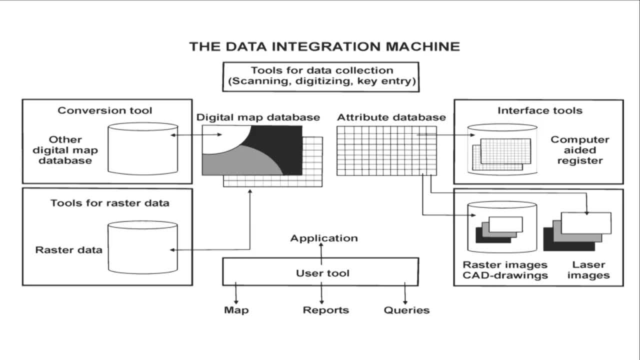 And, finally, you start creating applications, output in maybe form of maps, maybe in form of reports or maybe some queries, ad hoc questions. you raise to the. there is a question. Go to the system. you raise a question that I want to like in Google Map. 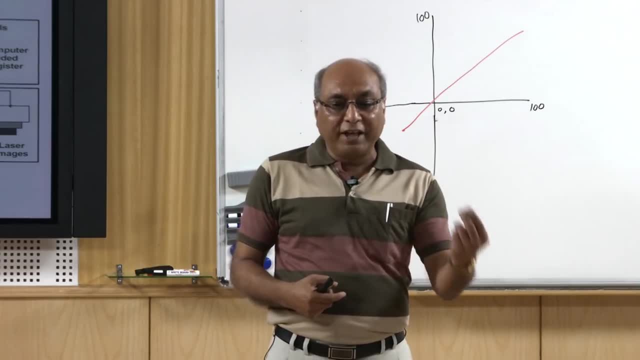 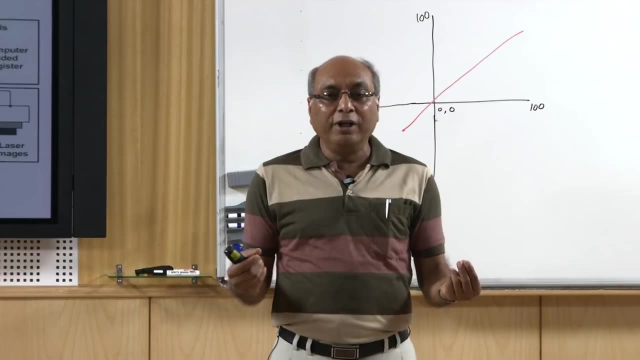 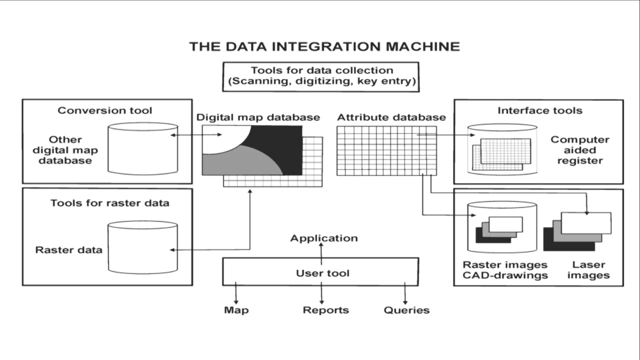 You, you indicate to Google map: This is my origin, This is my destination, And then you also indicate my mode of travel. So if you are traveling by road, it might provide different scenarios and therefore the queries, as per the user. define the specifications. 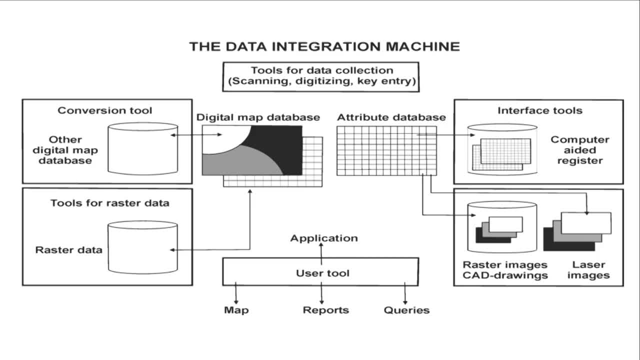 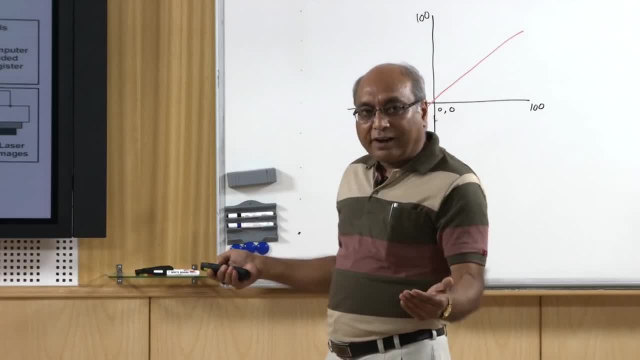 So a user has defined- has already defined- destination, origin and the mode of transport, And then, as per the user define the specification, theger can easily leave it andAMO access to Google. Oh cool, Ohkan. as per the your query, your answers are coming through map, as well as a report saying that. 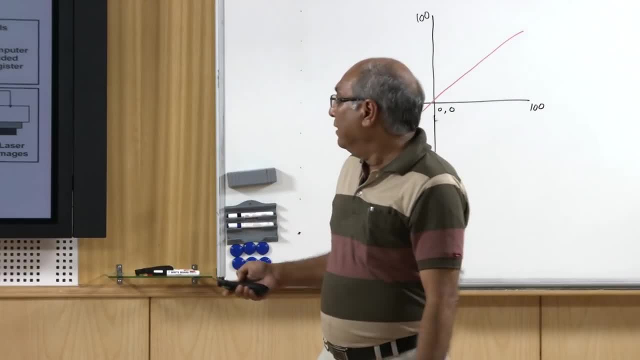 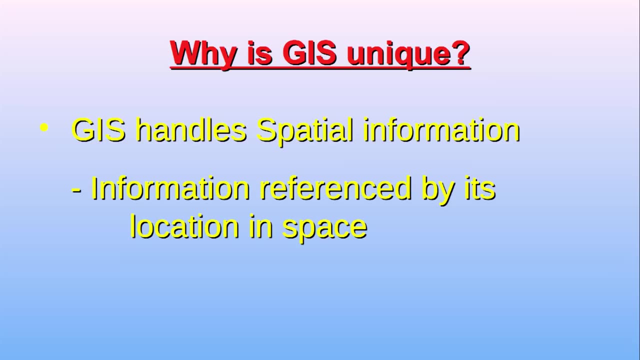 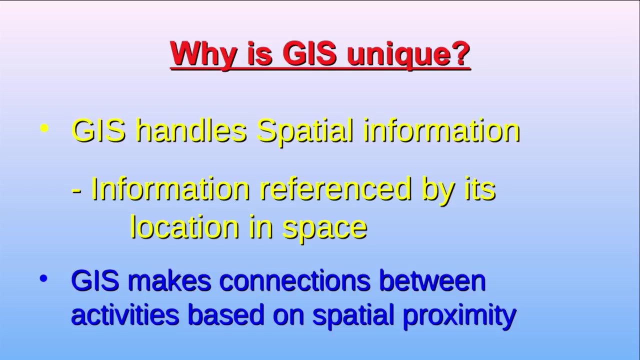 this is the distance, this much time it would take. likewise, so let i am coming to the end of this particular small lecture- is: the gis handles spatial information, information, reference by its location in space, that too, in geographic coordinate system. gis makes connections between activities based on spatial proximity. spatial word is very, very important and this is spelling. 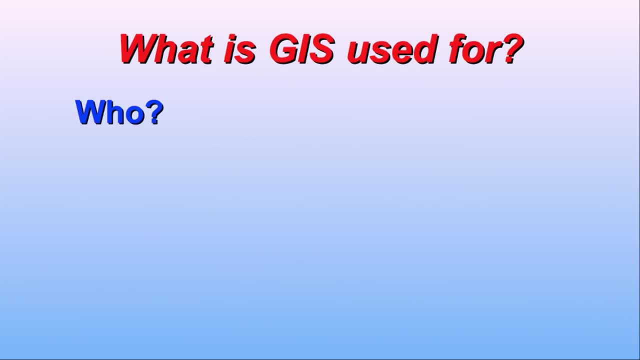 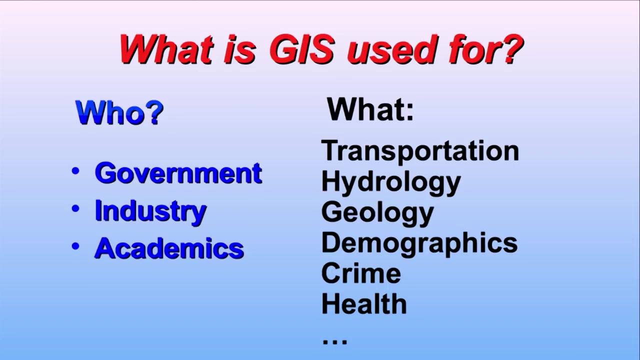 is correct. this is not a spatial, but spatial and gis who. who can use gis? a in government, industry, academics, even private people can use gis and what basically the questions? or which areas where gis can be used, like in transportation system. i have given the example. 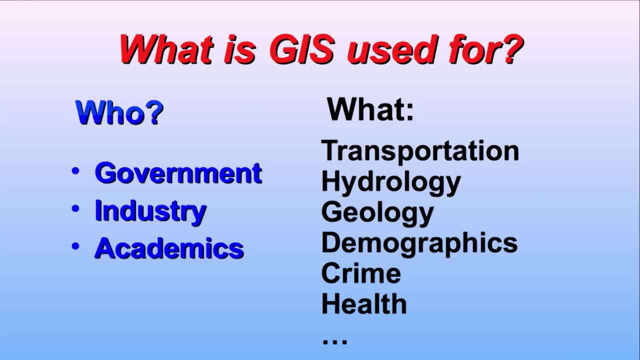 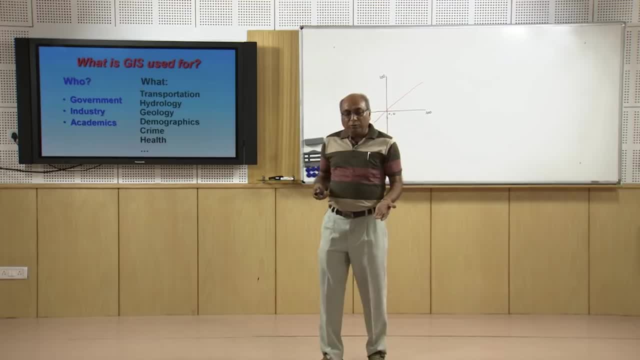 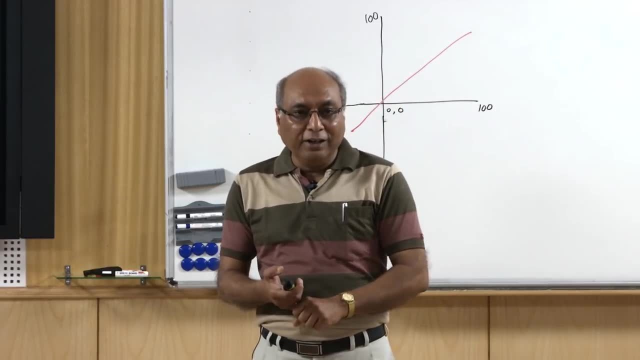 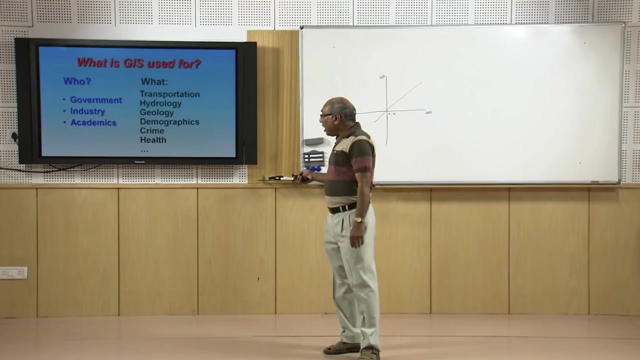 of navigation, in hydrology, ground water hydrology. in geology, in demographies, crime, health. in demographies, like census, department of government of india has started using extensively the gis. similarly, railway- indian railways- have started using gis extensively. so not only the government department, private departments are also using even the police, in some in big cities, police. 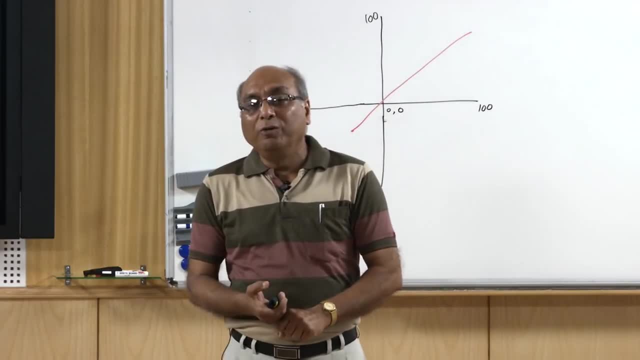 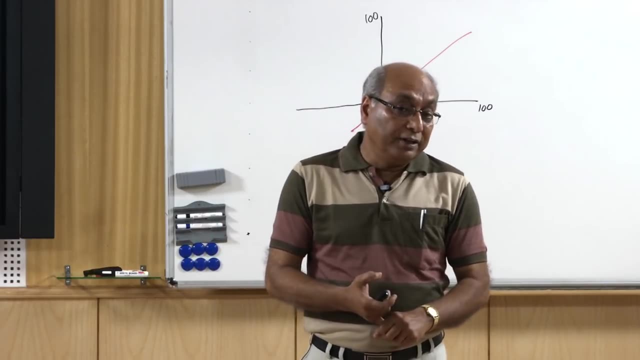 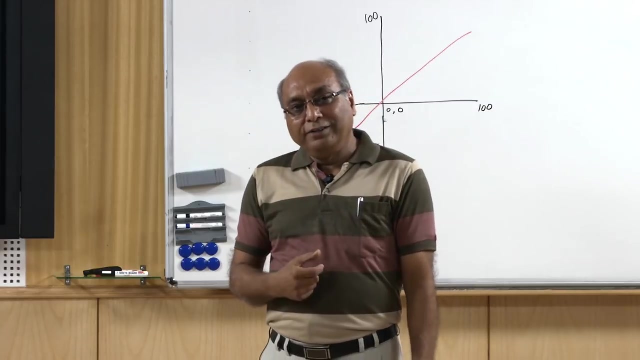 have also started using gis and in private units. So private, you know many taxi operators which are having hundreds of taxis in their fleet. they too are using not only the mobile technology but gis technology in integration. So the operator of those taxi fleets exactly know where is a taxi lying, ideal and once. 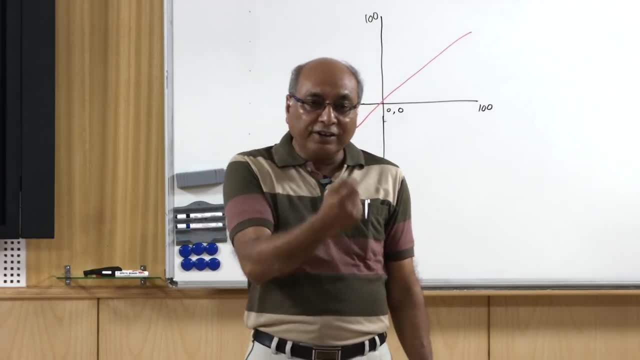 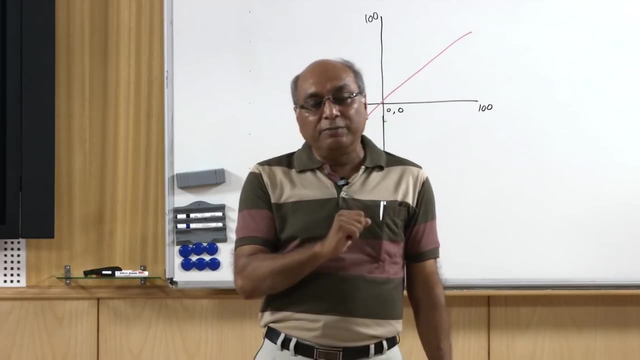 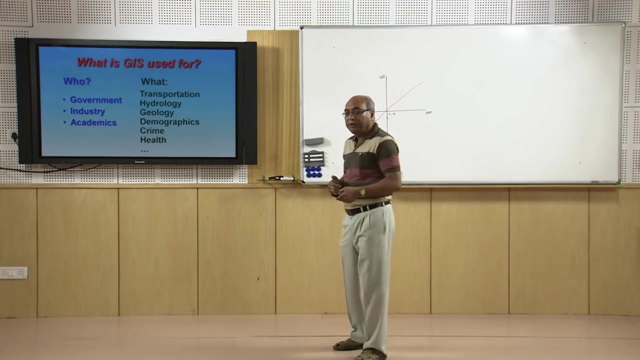 that is, taxi- is located, a customer calls, the location of that customer is also plotted on the map and if the taxi- whichever is nearer to that customer- immediately get the taxi to get the message and that it reaches to the customer. that is the advantage of having information in geographic coordinate system and this is what the gis basically provides. 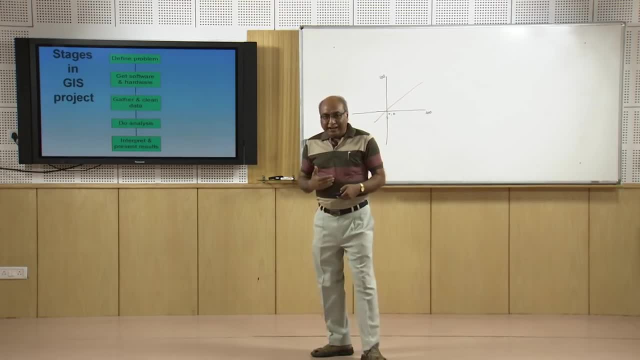 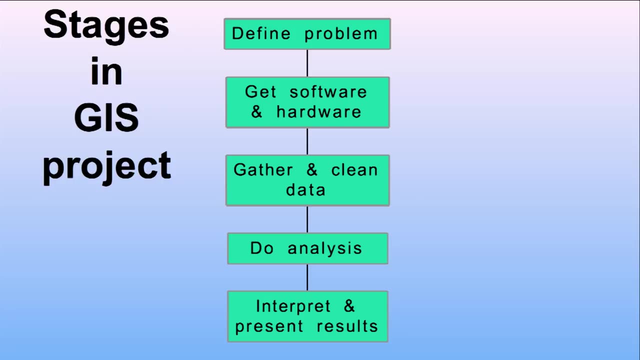 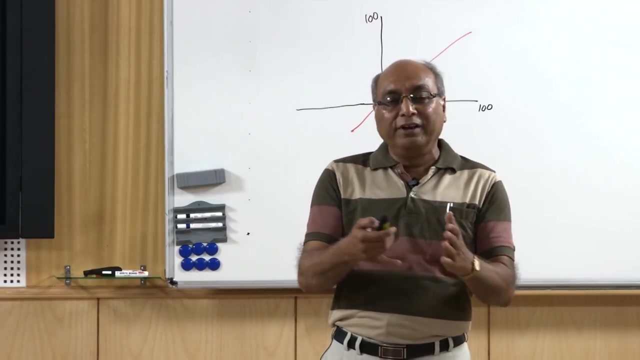 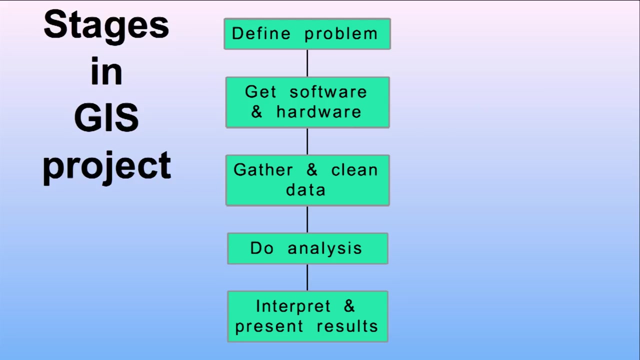 there are different stages in a gis project. in very brief, one has to first define the problem, the project, then get software and appropriate get software and hardware. there are hundreds of gis softwares, starting from free public domain, freely downloadable to commercial software. Very expensive softwares are also there, but very powerful. then gather and clean data. the